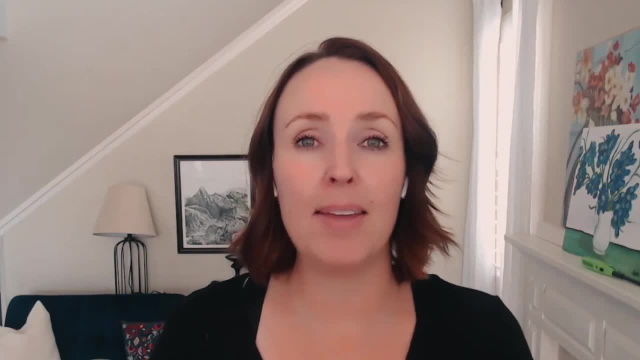 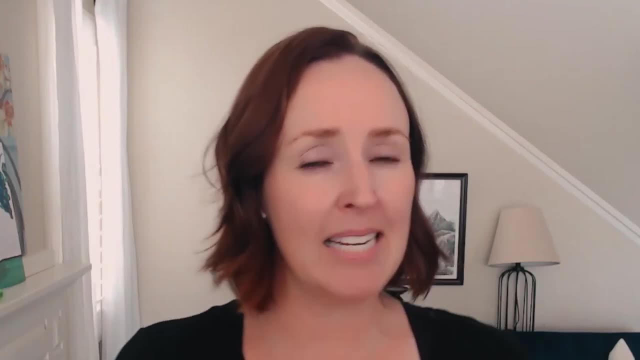 on the same continent or within the same area. I highly recommend that you get there early, And by early I mean at least a day, ideally at least two days, But if you want to build it into your vacation, then obviously you can come as early as you want to come. Luckily, none of our 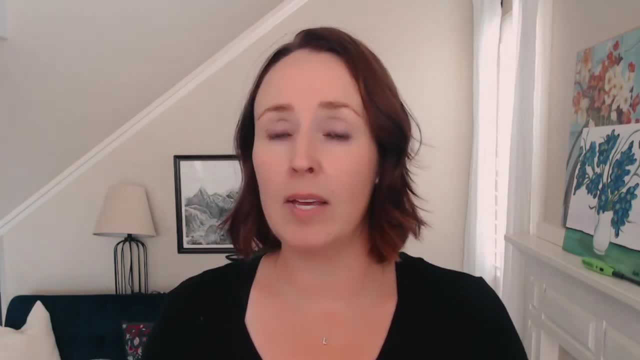 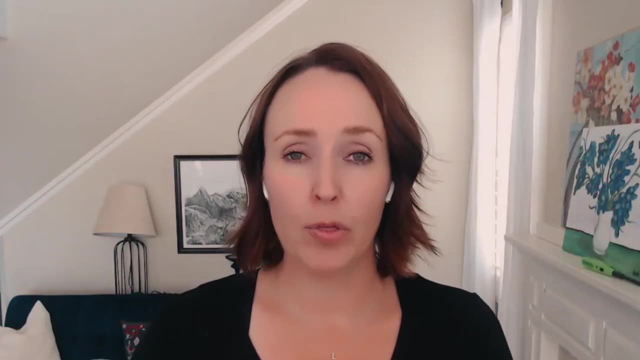 flights got canceled, But especially if you're going this year, flights are getting canceled and delayed left and right. So if you're going to Australia, New, Zealand, Australia, New Zealand, it's even more important that you get there early, just in case there's a cancellation. 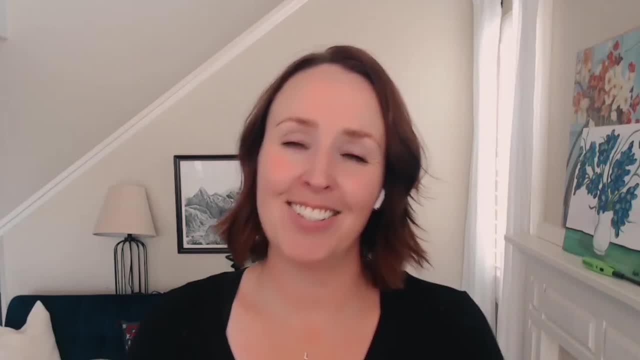 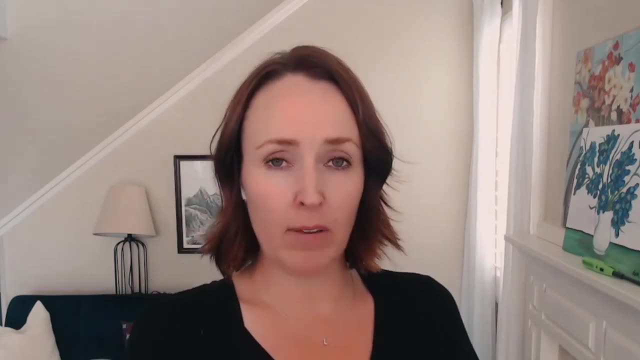 a delay, something happens. You don't miss getting on your cruise, So get there early. The cool thing about that is you can also build it into your vacation so you can explore that city that you're leaving from and be able to extend your vacation a little bit and give you 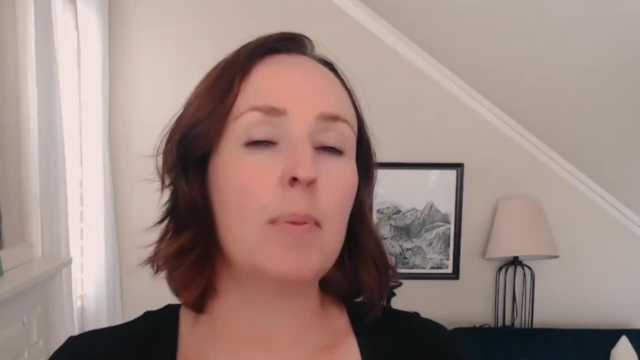 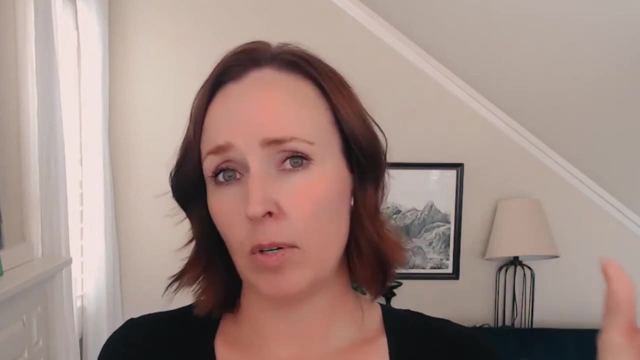 a little bit more in-depth of that particular city, Because the one thing about cruises is it's really just snippets of each city. You're only really there for eight hours, 10 hours. If you're lucky, you might be there overnight, But for the most part 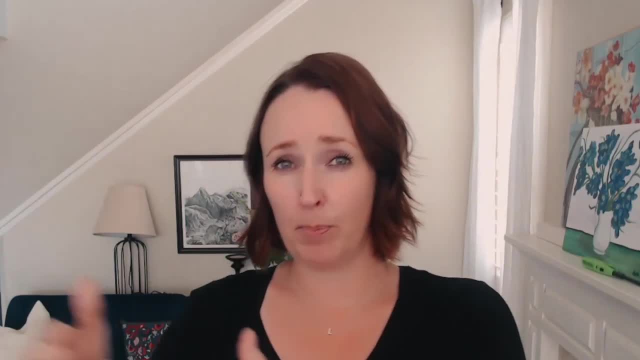 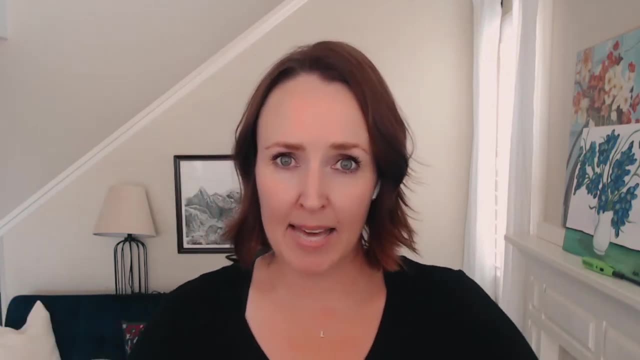 you're only in each city, tiny, tiny little bit. So if you can extend the beginning city and the ending city, all the better, because you can get a far more in-depth look at those cities. All right, Speaking of arriving and getting that whole thing going, I also highly recommend that. 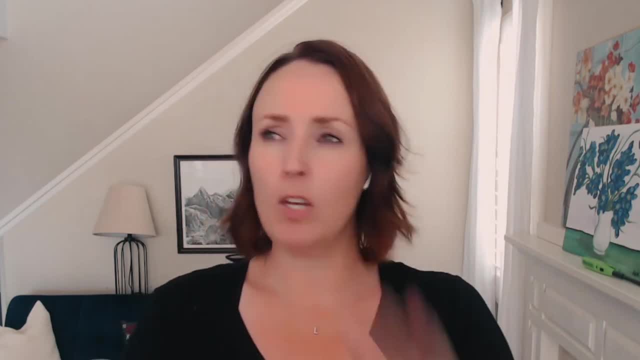 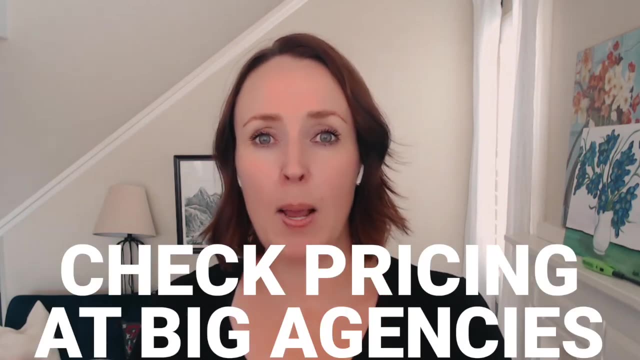 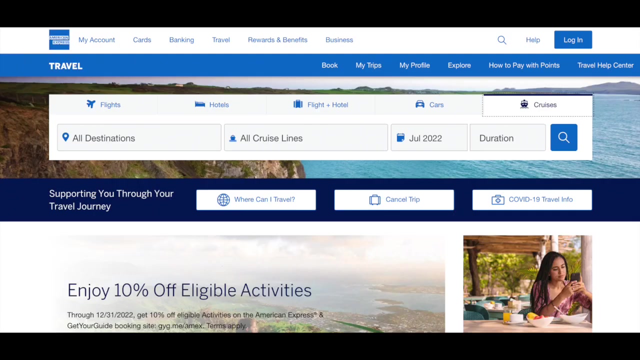 when you book your cruise, make sure you and you might want to book it yourself through the cruise line directly, but I highly recommend that you also check with a big travel agency or or someone affiliated with a big agency. If you have an Amex card, check Amex If you belong to. 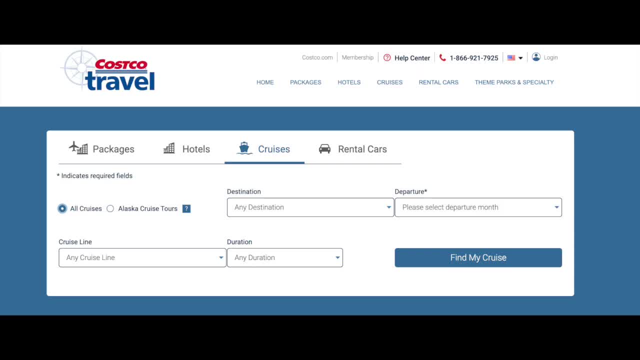 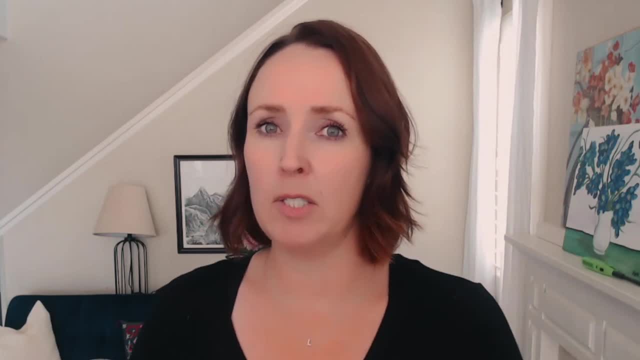 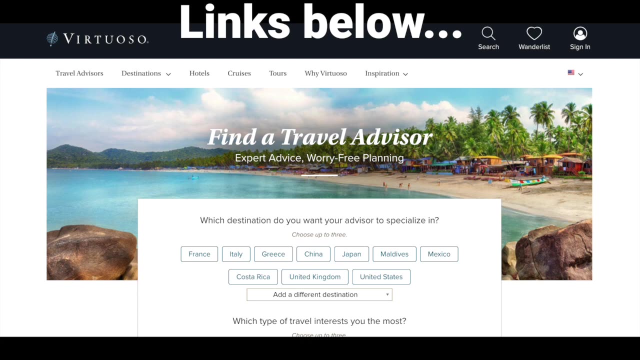 AAA, check AAA or Costco. If you have Costco, check Costco. And if you don't have any of those, then find a travel agent who's affiliated with a big travel agency. There are little home-based travel agents that belong to large consortiums and large agencies that can have access to what I'm about to tell you Now. the reason why I want you to check these big, large agencies is because they have more buying power, more negotiating power with the cruise lines. So oftentimes, when you book through them, they will give you extra perks. better than what? you're finding by booking through the cruise lines directly. So you'll get extra room credit, You can get discounts, You can get upgrades, You can get extra amenities in your room- all sorts of things that you can get by going through a big agency, because they have these. 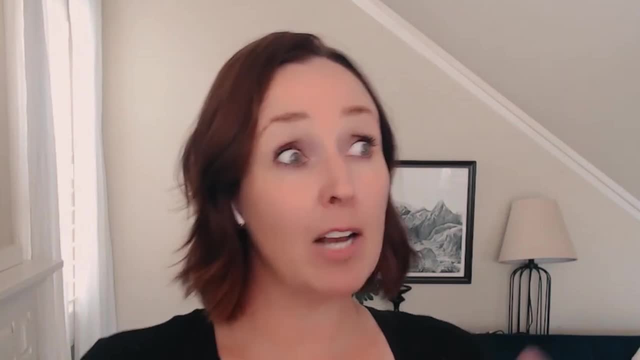 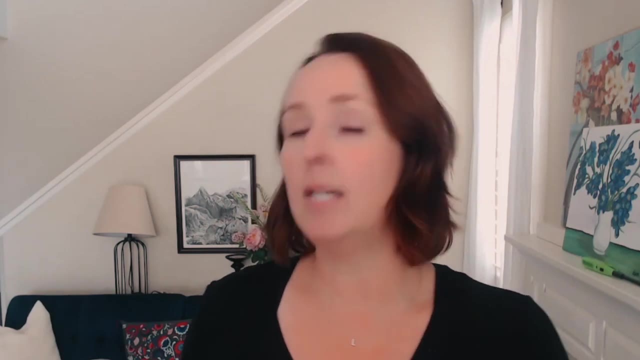 packages that they're allowed to offer you, These extra extras that they're allowed to offer to you. So, for instance, we booked our cruise through American Express, their travel agency, and we got extra room credit. I think we got an extra $500 in room credit. 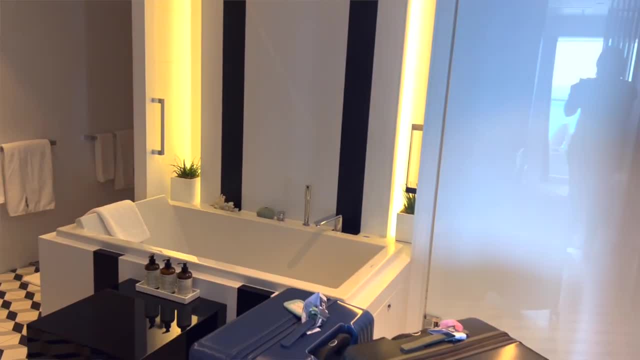 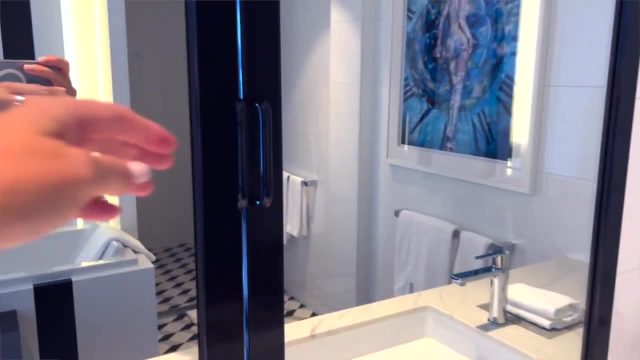 We got a bottle of champagne when we arrived, And then I think there was one other, I think there was an upgrade that we got as well. So it was by far worth it to check- at least check with those big agencies- and see what extras you can get and be able to take advantage of those extra. 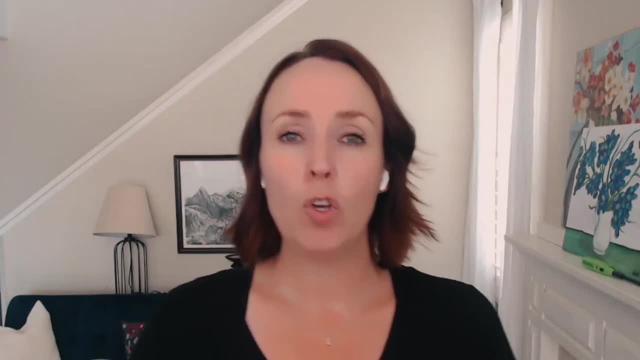 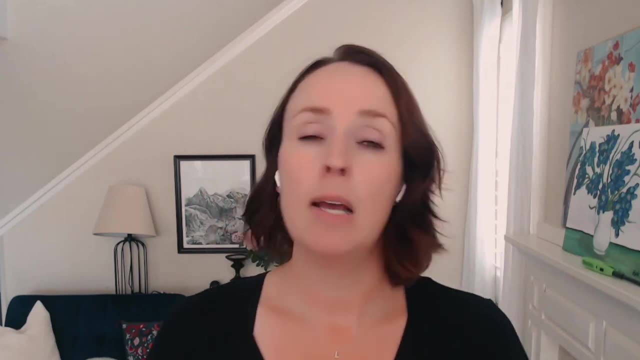 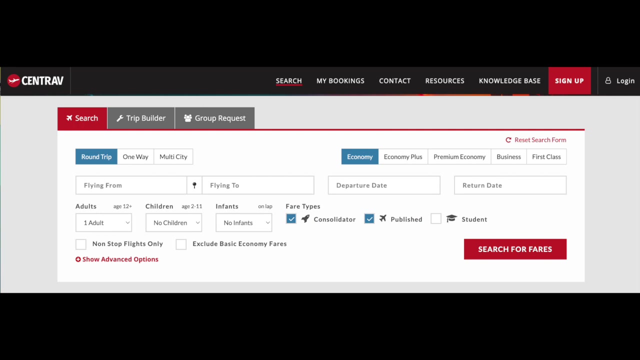 opportunities. On that note of booking things when you are pricing your flights, to get there I priced all of the usual places that I recommend people price their flights. I went to Google Flights. I went to some of my old travel agency. friends have access to some of those consortiums and things that I could book flights through. I checked there, I checked with the flights directly, I checked everywhere And I kept finding the same basic pricing structure. For some reason I was hesitant to check through the cruise line. But one day I was fed up because I wasn't finding what I was looking for, And I was 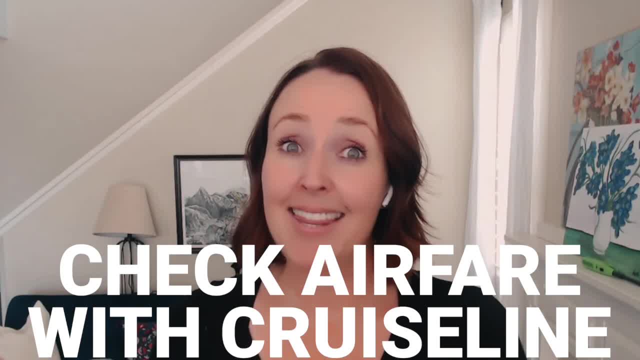 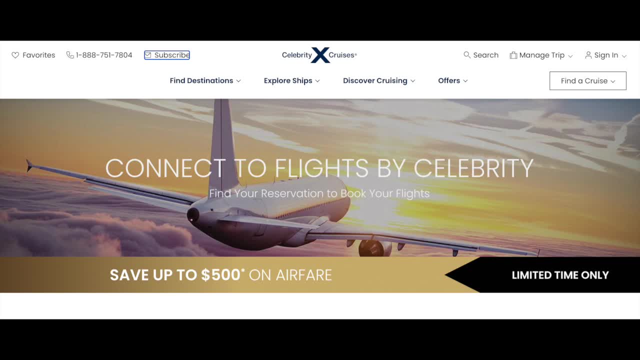 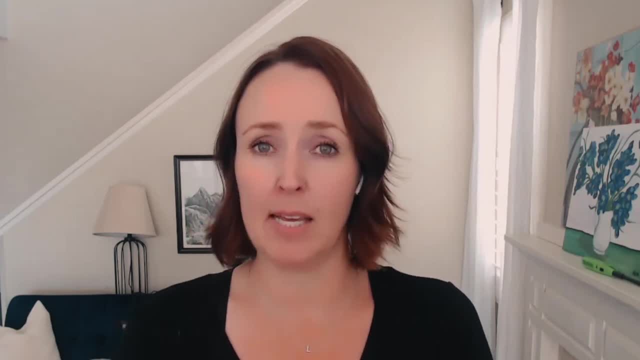 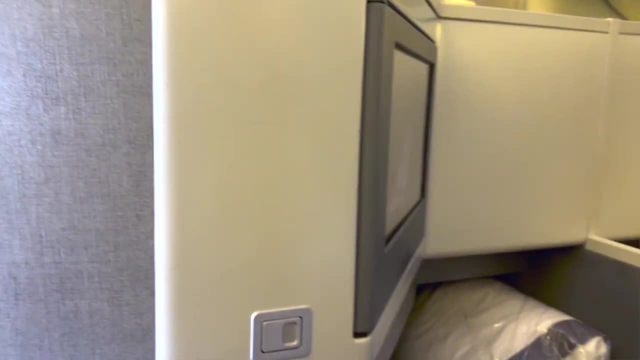 available to while we were traveling, for any emergencies that came up during travel, which I have a story to share with you in just one second, And because they saved us money. we were able to upgrade our flight and fly business class, which I'm telling you if you're going to Europe. 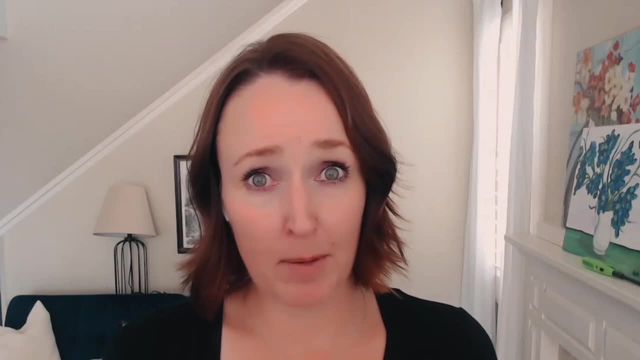 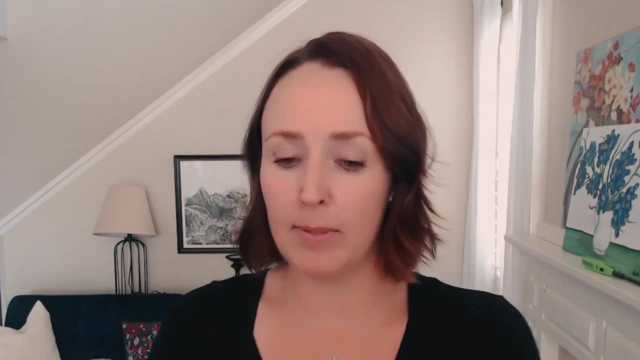 especially from far away. it's definitely worth it to get business class when you're traveling 20 some hours on the flight. So by going through the Air Department in Celebrity I was able to do those things. Now the story I was going to tell you. So they do offer help. 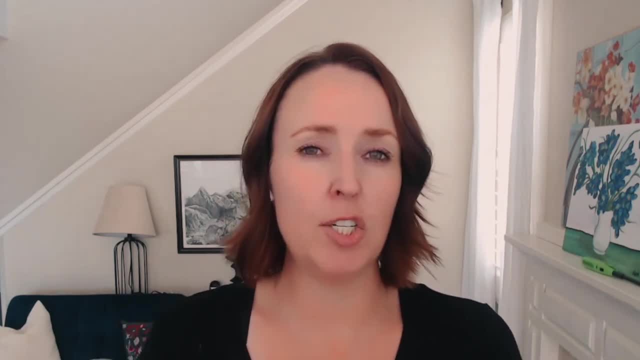 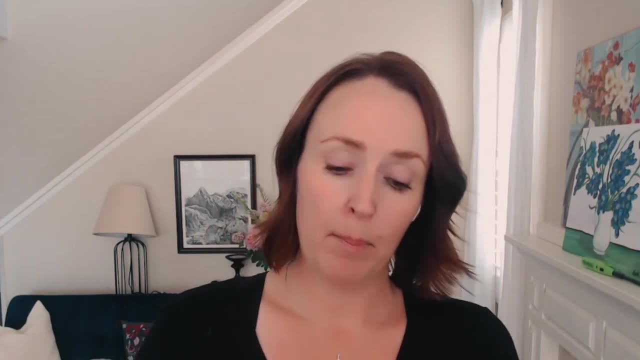 during your flight. So if something is canceled, delayed, something changes, you can call them 24 hours a day and they will help you fix it. So when we were coming home, my daughter's flight- we ended up on different flights and my daughter's flight was delayed. 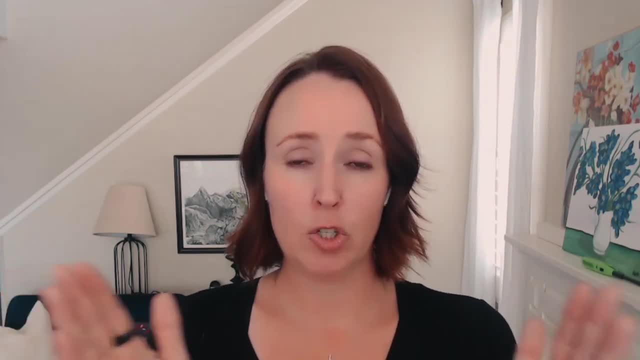 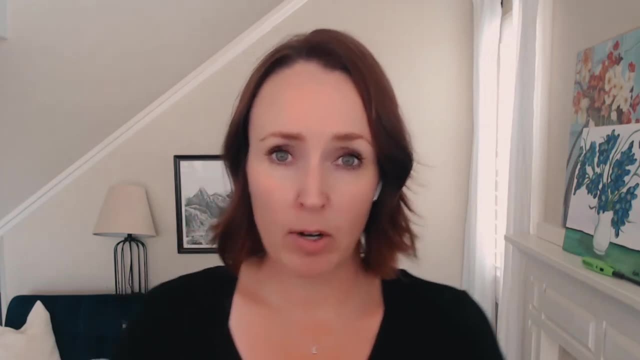 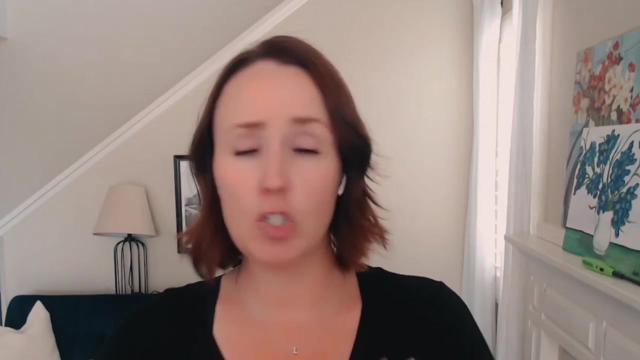 leaving. It was delayed a few hours, But by doing that it shortened her layover so they would miss their connecting flight, And so she was able to call the Air Department and they immediately fixed her on a totally different flight that was nonstop. They just took care of it for her. So I highly 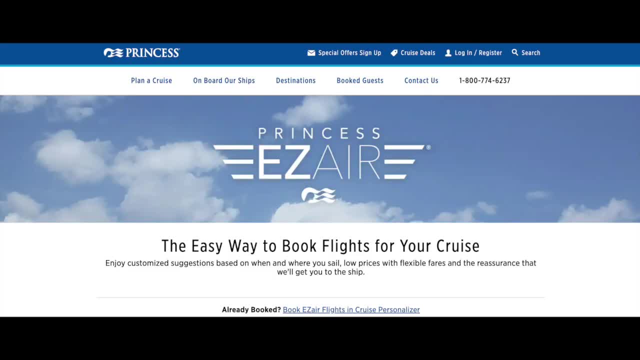 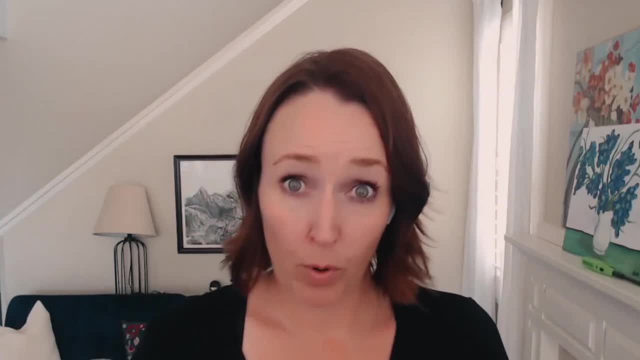 recommend at least looking through your cruise line's Air Department and see what it is that they offer, Because by booking it through them, you might have some of those extra perks that might make it worth it for you. Now, if you don't book through them- and in general, I highly 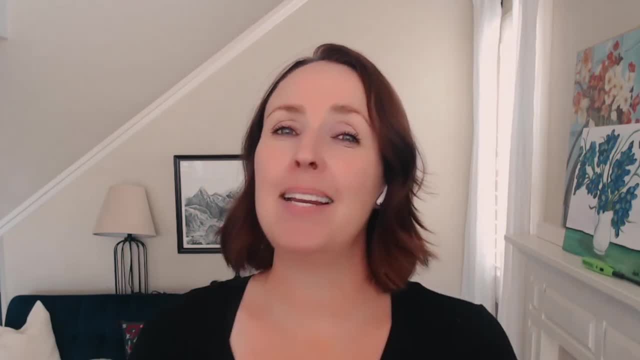 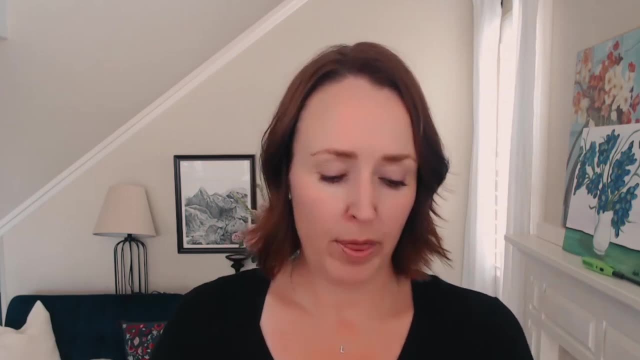 recommend always get travel insurance. That is my next tip and kind of a bonus tip because I don't have it on my list. But my bonus tip is to get travel insurance. especially right now, with a COVID coming and going at a whim, You never really know we're monkeypox or anything. 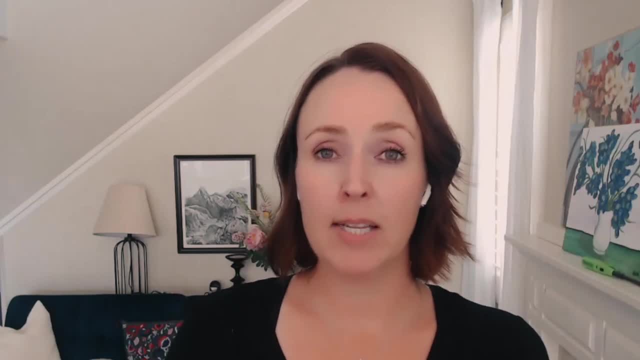 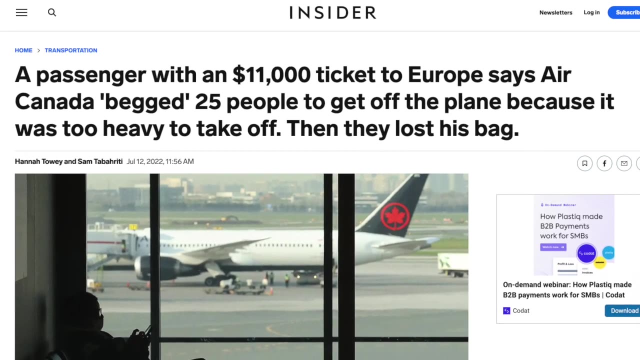 else going on right now, But also all the cancellations and all the delays. If you find yourself in a situation where you're canceled, delayed, your baggage gets lost because they moved you to a different flight and they didn't bring your baggage along, or whatever happens. 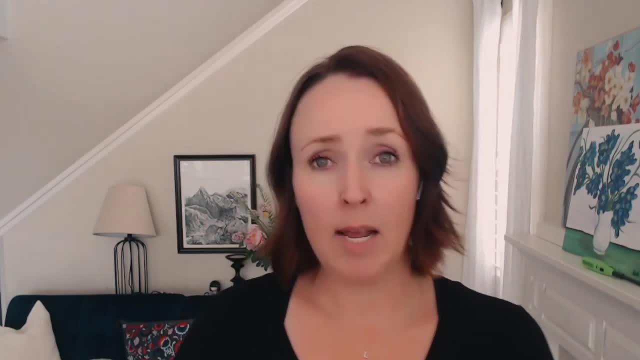 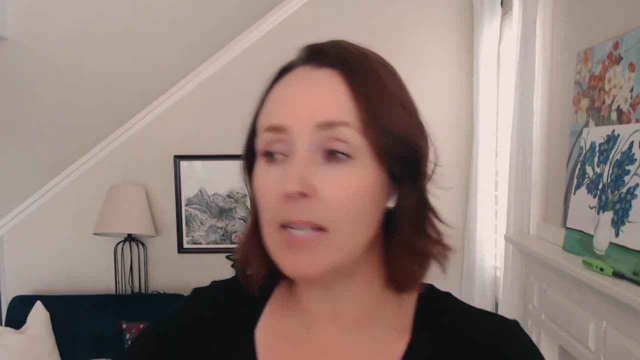 or you're traveling and you lose your money, your passport, your ID, then travel insurance will help protect you. They will help you make those new arrangements. They will help give you the money if you need money to make those new arrangements. They will help you get your new passport. if you lose your passport, Sometimes they'll even give. 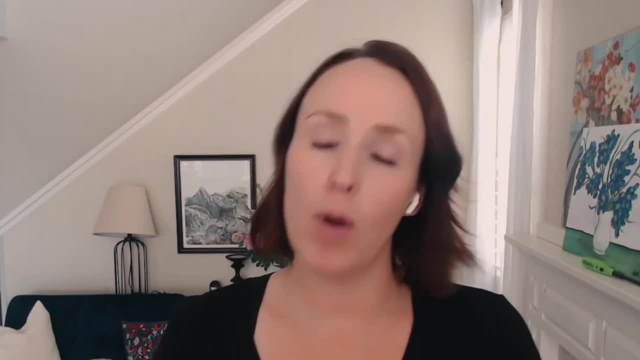 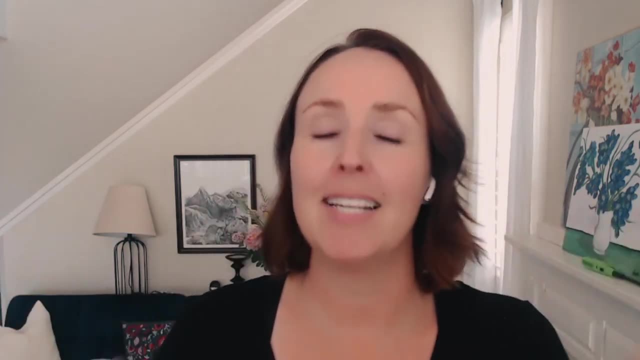 you cash if you get pickpocketed and take all your cash. So I highly recommend travel insurance, regardless of if you get air through the cruise line or not. Always, always, always, get travel insurance. My next tip is picking the right cruise line for your needs. So cruise lines: 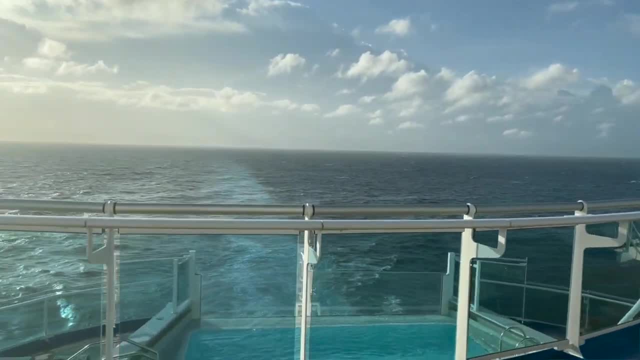 if you don't know already, they're similar to hotels in that if you're going to a three-star hotel, it's a certain level of service, a certain level of amenities, and you're going to need a cruise line. So if you're going to a three-star hotel, it's a certain level of service, a certain 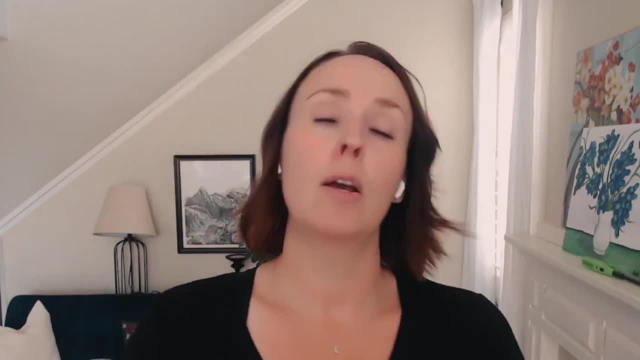 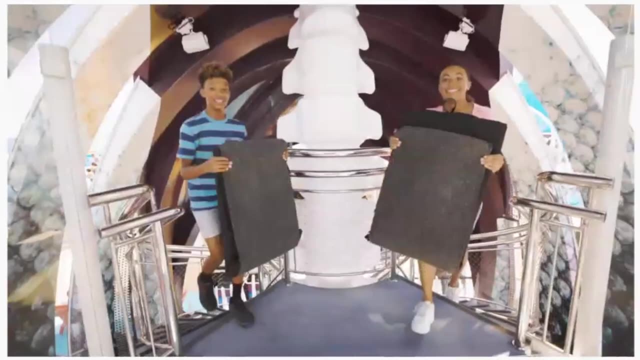 level of amenities and things that you expect. same thing with four-star versus five-star Cruise lines are the same. You have your mast lines, which are going to be like Carnival, Royal Caribbean. They are going to be more crowded. They usually have 4,000 to 6,000. 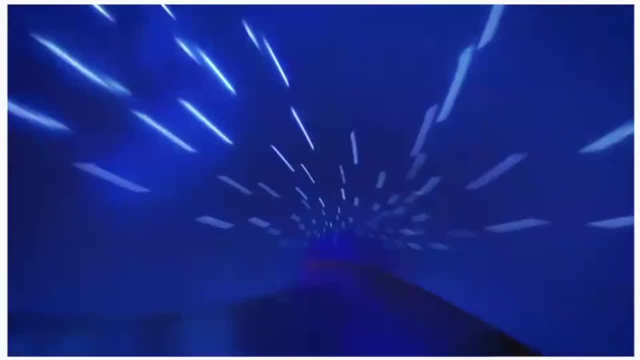 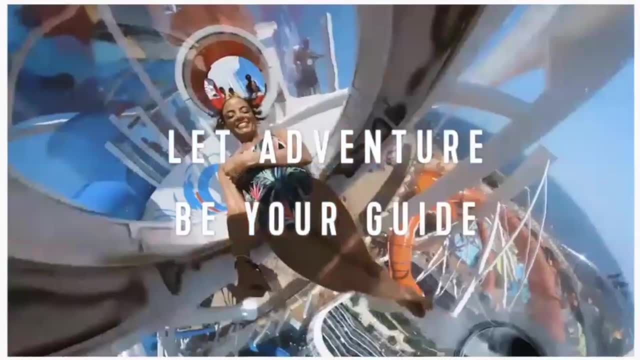 passengers on board, so far more crowded. They are going to have a ton of activities. These are the ships you see on TV that have water slides and ice skating rinks and zip lines and surfing off the back, the Flowrider things. Those are those ships. Those are what those are going to have. 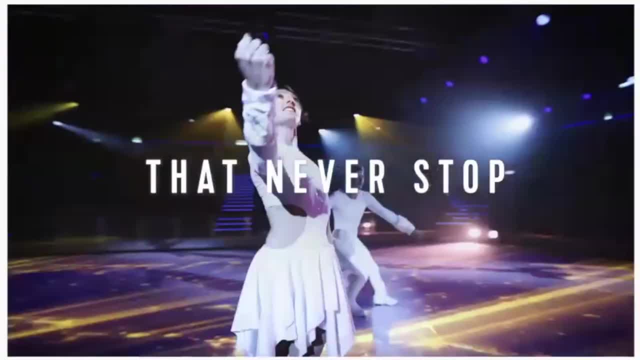 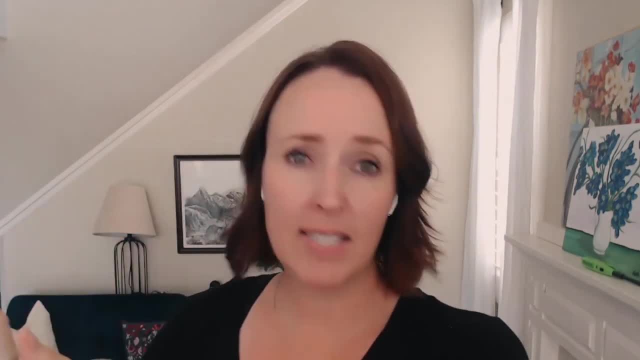 But again, by having far more people, they're going to be a little cheaper and they're going to be a little more crowded and a little bit less service. But if you're traveling with kids and family and you want a lot of activities, fantastic, fantastic. If you are kind of wanting a little bit. 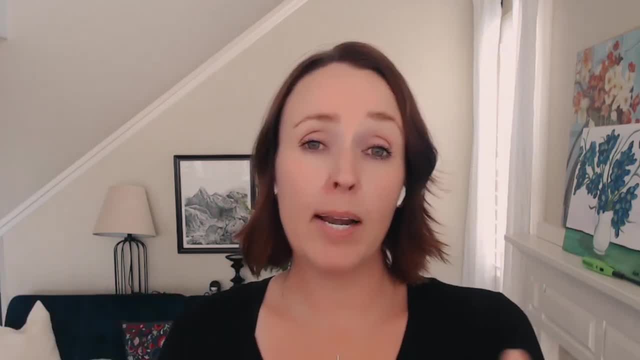 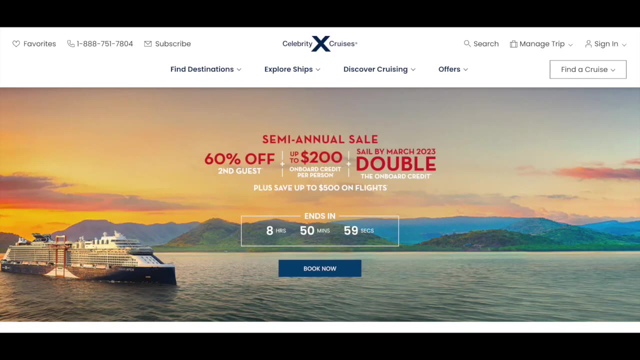 more service, a little more luxury, a little more upgrading as far as the food, the rooms, the amenities, things like that. then you're wanting to go with the premium class. Premium class is usually where I choose to cruise and that is Celebrity Princess Holland America. but 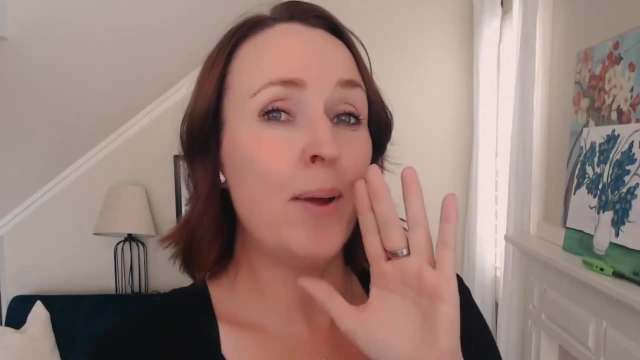 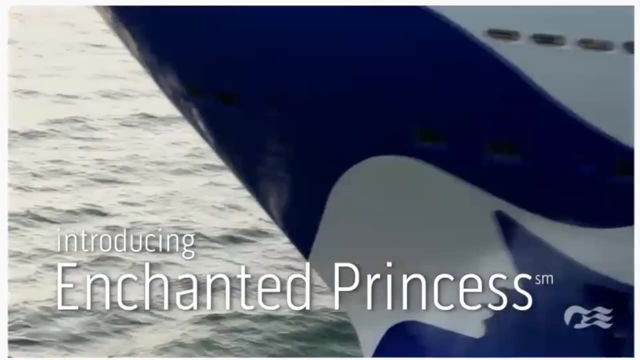 Celebrity and Princess are my favorite. I don't like Holland America, but if you're a Holland America lover, more power to you. That's the premium class. You're not going to have the water slides and stuff, but you will have beautiful pools. You'll still have casinos. 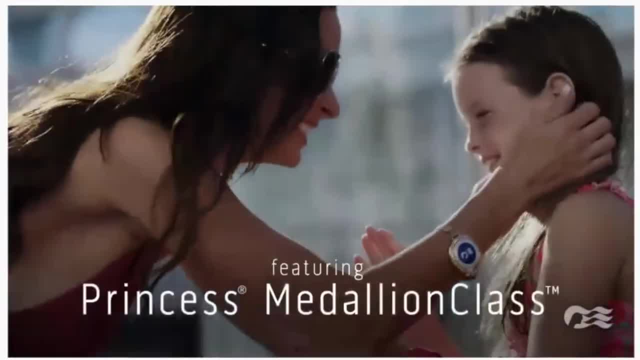 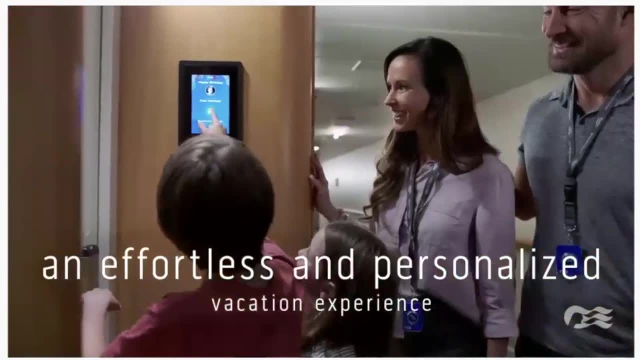 You'll still have Broadway-style shows and things of that nature. So you'll still get some of those amenities, but you'll get less people: closer to 2,000 to 3,000 people instead of six. There's usually more staff per guest, so you get a little bit better level of service. You get a little bit. 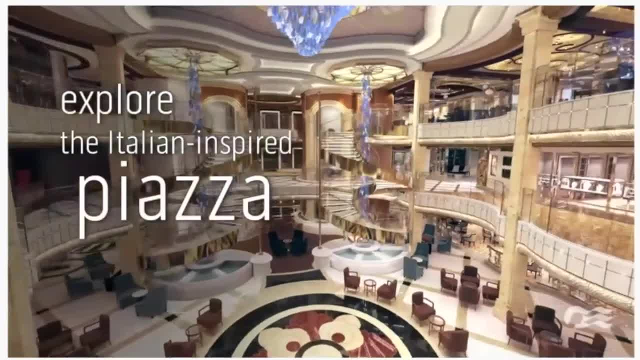 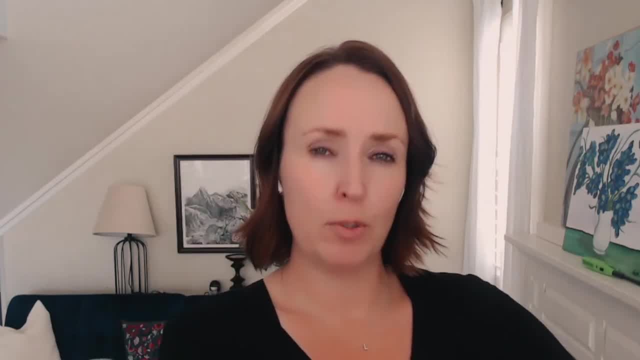 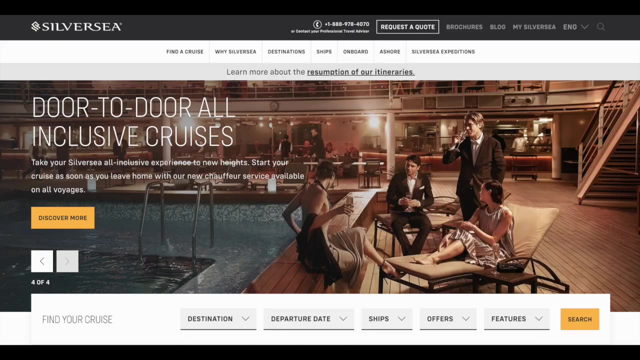 more level of food and it's just a little bit more luxury all the way around, And then if you are a luxury traveler, then you want to go to the higher level. This used to be Crystal, who's no longer in business now, although I heard somebody is going to buy them and restart them, But this 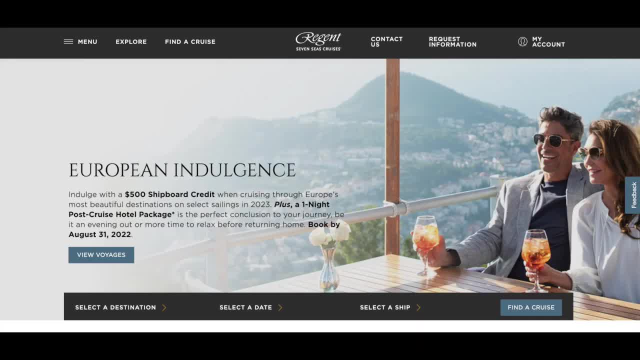 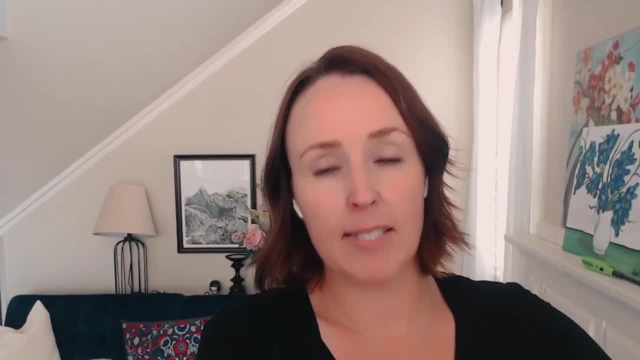 is going to be your Silver Seas. This is going to be your- oh, I'm blanking on the name. I can't remember the name. I'll tell you some of the names, But these are going to be your super luxury lines. You're going to have far smaller ships, far smaller. You might only have 700 passengers less 1,000 passengers. You're going to have far more staff per person. It is going to be luxury, like staying at a five-star resort, like staying at a Four Seasons or something of that nature. 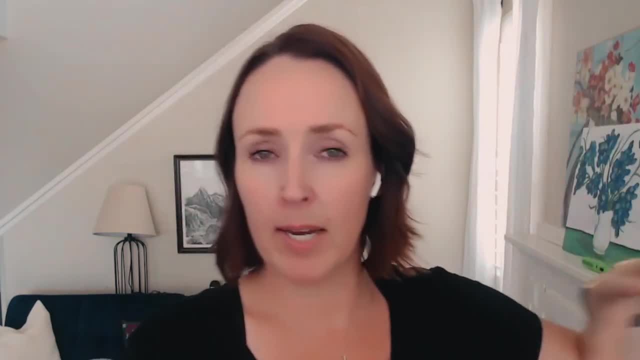 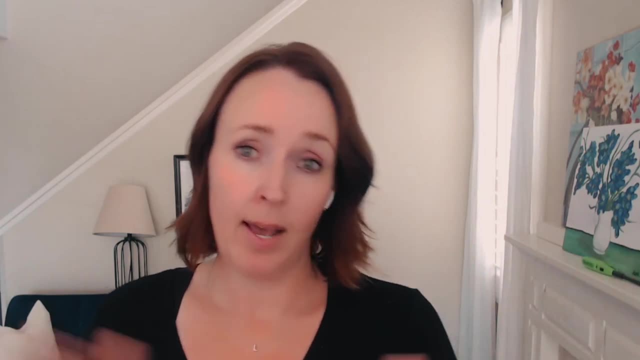 It's going to be much higher on your food, your service and just the quality of what you're getting. It's a far more luxurious cruise. When you go to the Mediterranean, think about the experience you want to have and then choose accordingly, And then go book it with one of 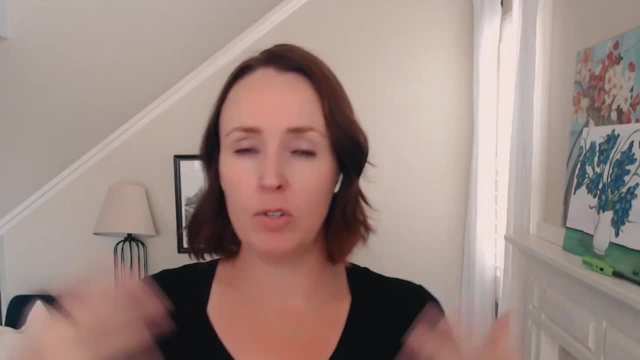 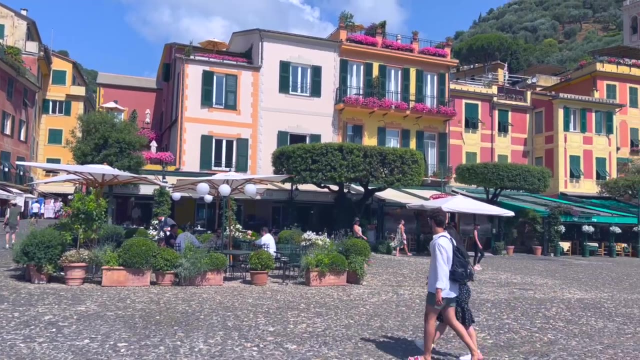 those big travel agencies That can give you lots of perks. So now you are on your cruise. You're exploring the Mediterranean. One thing that you want to remember is: these are just snippets. They're just tiny little bites of these cities. There's no way. 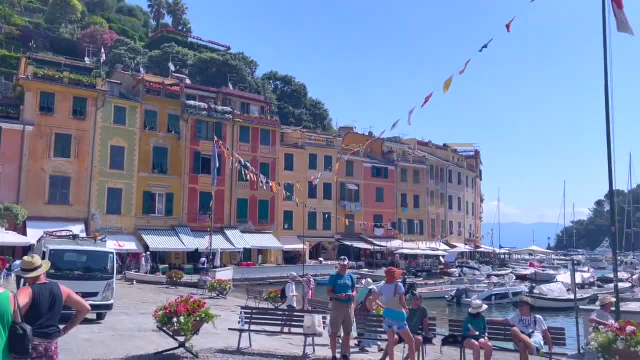 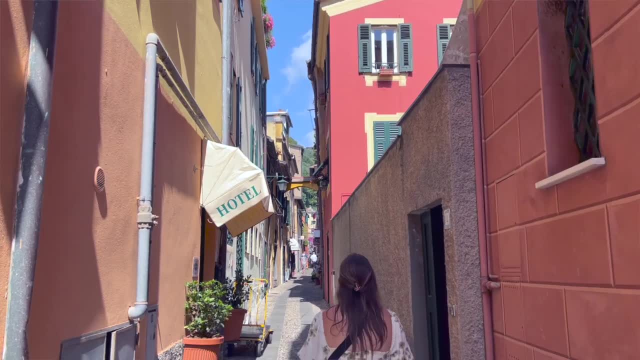 you're going to be able to explore Florence to the fullest: Pisa, Rome, Cannes, Paris, anywhere that you're going. Paris technically isn't the Mediterranean, but you know what I mean. You're not going to be able to explore each of these cities in probably as much as you would. 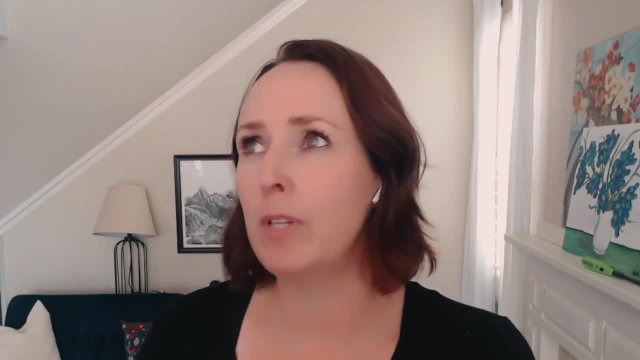 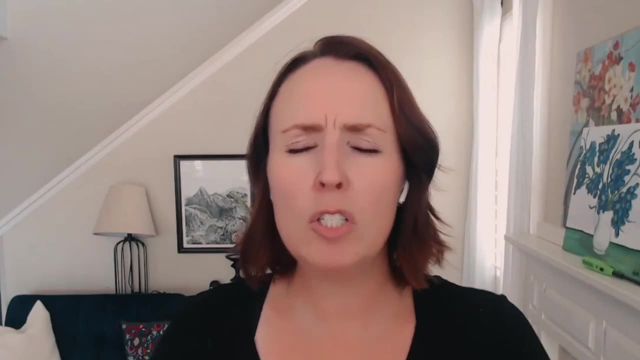 like to, because when you go to these cities, they're gorgeous and beautiful and amazing and if you've never been there before, you want to see everything there is to see. The only downside is there's a minimum amount of time, So just know that, going in knowing 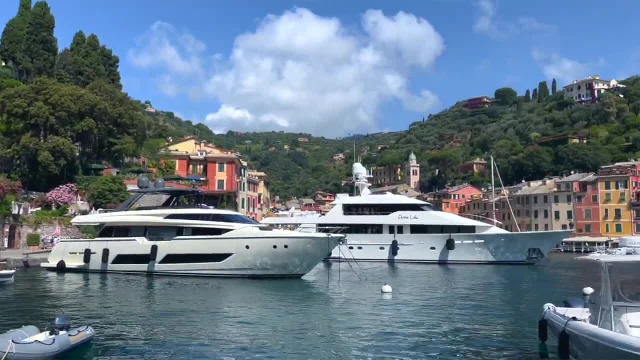 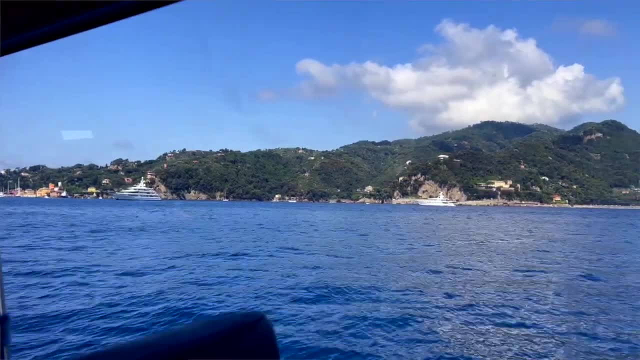 you're only going to have a little brief moment in time, don't try to fit everything in. You're going to be exhausted and it won't be any fun. Just pick one thing you want to see or explore or do and do that and enjoy it and love it, And then just make mental notes of all of the places you 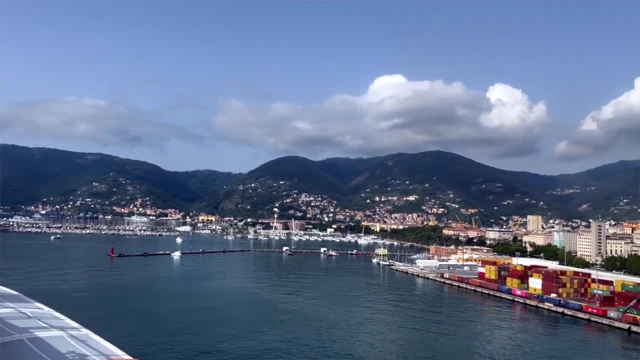 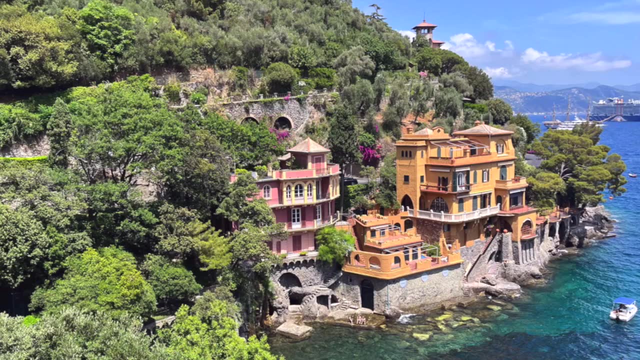 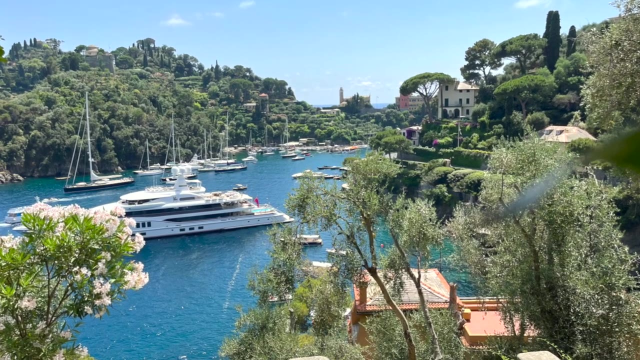 love and then go back another time and actually stay in that location for a little bit longer so you can enjoy and experience it all. One of these places that I absolutely loved is Portofino. It was gorgeous and amazing and it was tiny, so you felt like you could see it all. But, honestly, 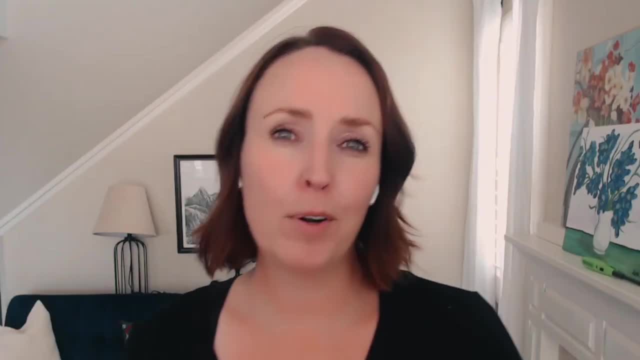 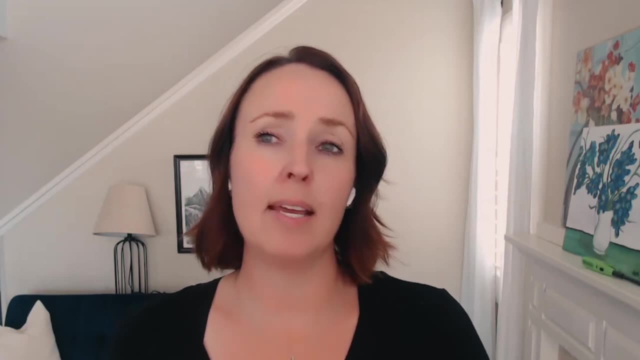 it doesn't do it justice. It's just a taste. So we will go back later to explore Portofino and some of the other little cities along the Mediterranean. So just know that, going in and don't think you're going to see everything and do everything, It's just going to be like 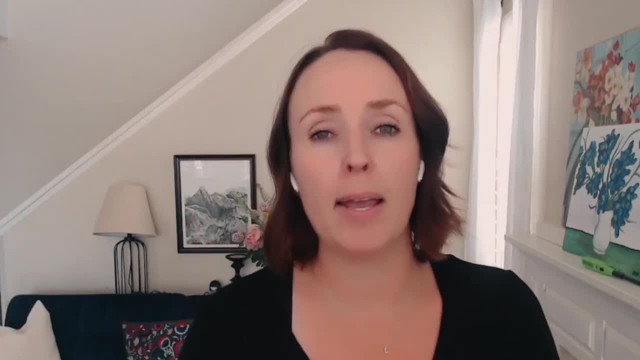 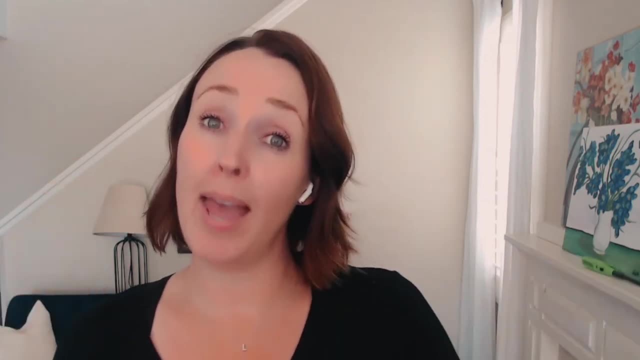 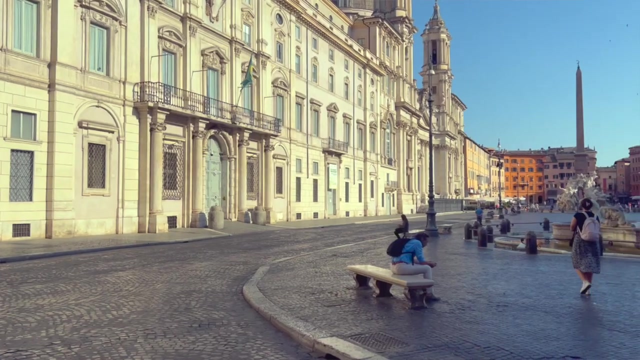 a sampler platter and you're just going to sample them and then plan another time to go back and explore the places you want to go. Now, the caveat to that is obviously where you leave from and where you end, because those you can build on to or you can plan to come back to some of those places. 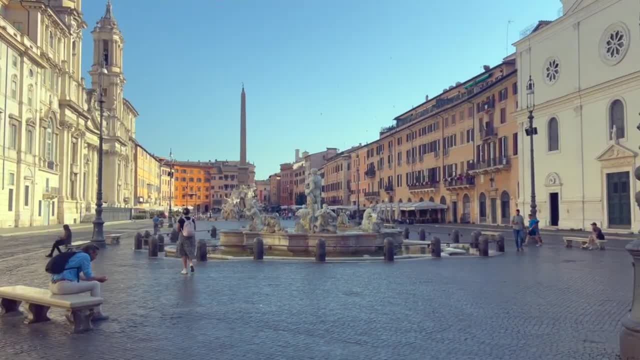 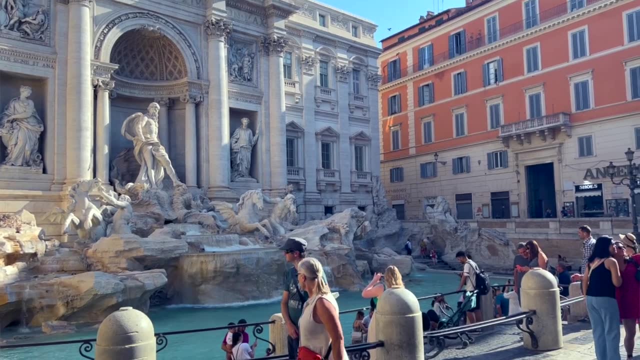 So I had already talked about adding time at the beginning of your cruise, but also you might want to consider adding time at the end. So for our cruise, we left out of Rome and we ended in Barcelona, Rome. I added days on and I'm glad we did because we got to explore. However, I didn't do it. 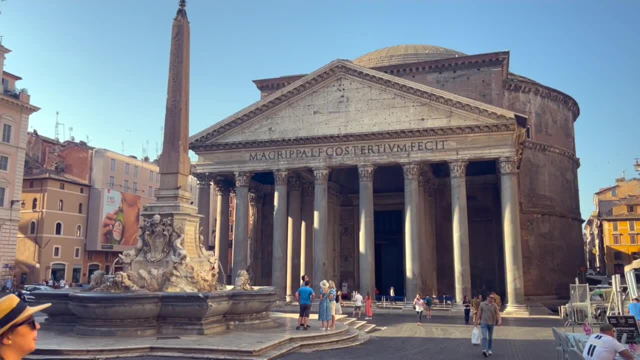 in Barcelona. I was worried by the time I got there that I was going to have to go back and explore. But by the time we got to the end we'd be exhausted and just want to go home. And now I wish I had. less time in Rome and added another couple days in Barcelona, so we could have explored Barcelona, because, as it was, all we did is drive through on the way to the airport and that's all of Barcelona that I got to see. So, if you have an opportunity, add time to the beginning and then to the end. so, that you can explore those cities in a little bit more in depth as well, And if you already know there's a city on your route that you want to spend more time in, perhaps add that on as well, And then either take a shuttle, a bus, a train, something down to that city or to that city, and add a little more time there. Just because you're on a cruise doesn't mean that's all you can do. Yes, it's a sampler platter, but you can always build it out and explore and add things at the beginning and at the end. that will make your trip just far more glorious. 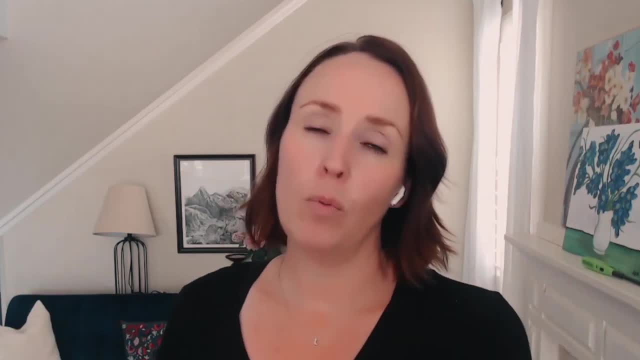 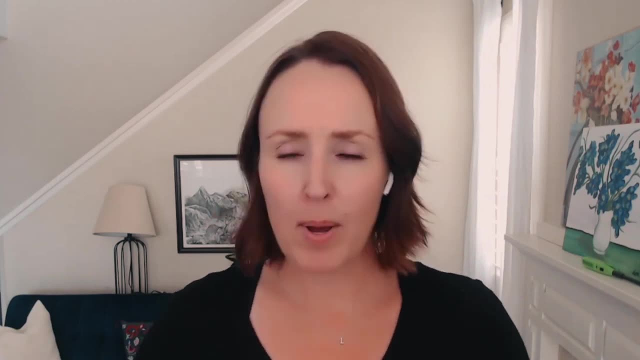 And especially if you're coming from far away, you don't want to waste the time and the travel that you've done and you really want to make the most of your European vacation. So think about that, Think about adding some things in the beginning and the end and making your 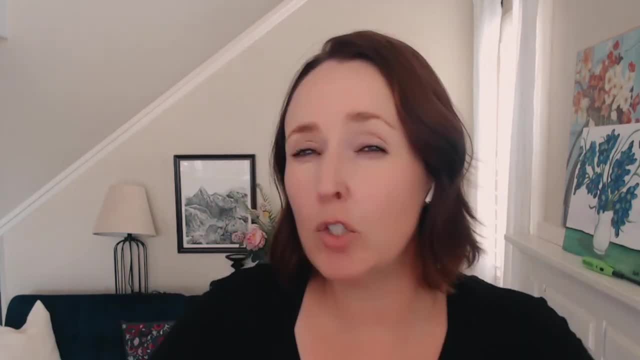 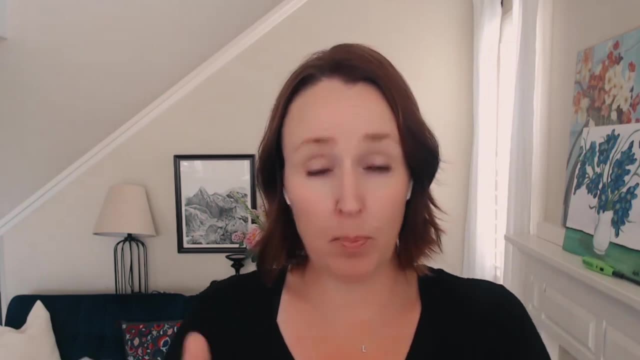 experience far more enjoyable for you. So, in regard to cruises specifically, you have shore excursions, And if you're not familiar with cruising is they usually have in each port that you go to. the cruise ship itself offers a variety of tours, activities, things that 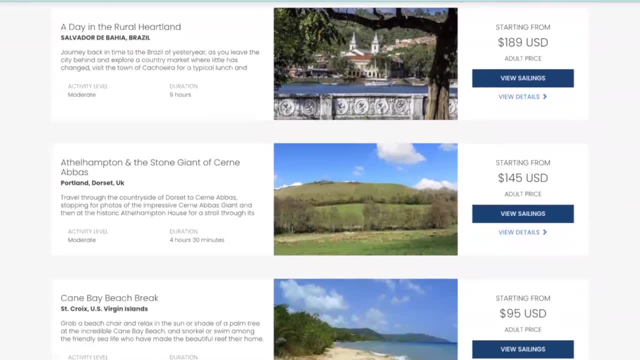 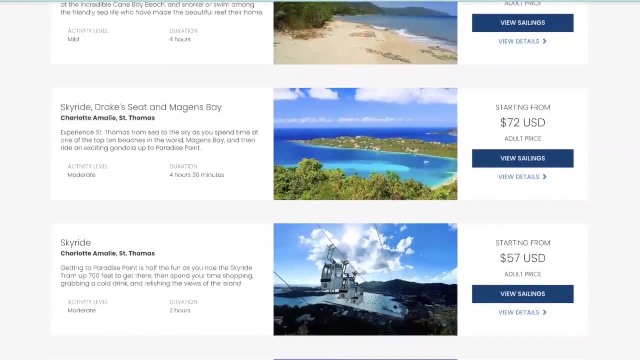 you can do sponsored through the ship. Now there are some benefits to this. A they keep track of it, so you don't have to worry about a tour coming back late and the ship leaving without you, Or you accidentally book something that starts before the ship even gets there, which has happened. 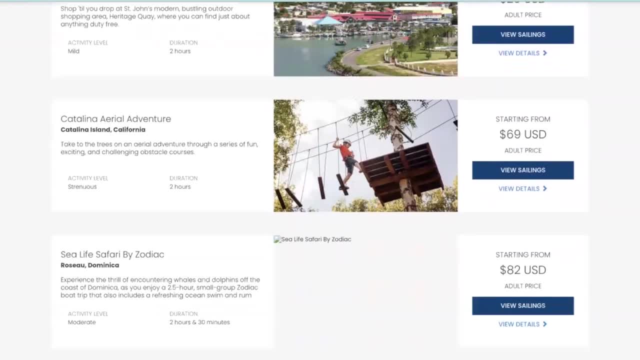 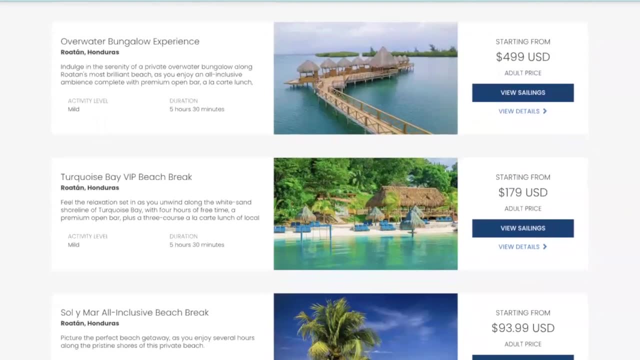 So they monitor things for you. They also vetted all of the tours and things so they know that they're safe. They're not going to put any of their guests on anything that would be not safe or potentially risky in some way. I personally will do them occasionally. 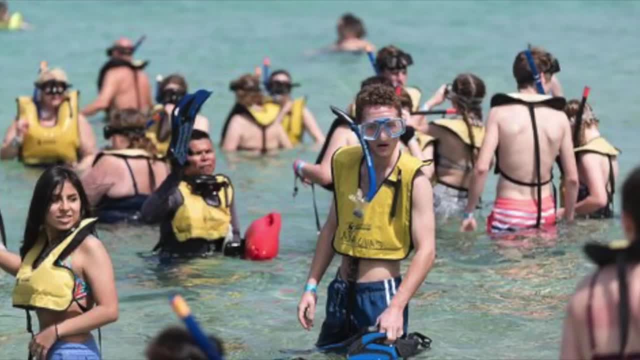 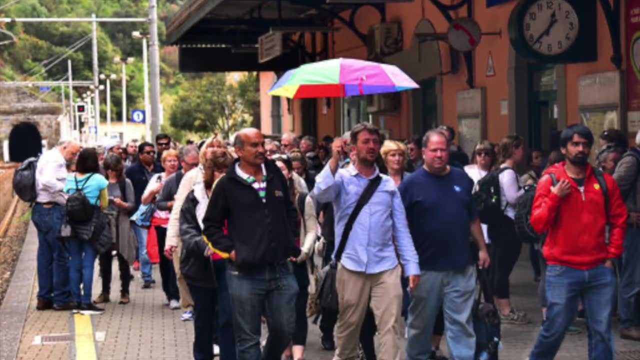 because some of the negatives of the shore excursions is they tend to be way overcrowded, way overcrowded, Even on those luxury ships. you tend to get a lot more people on your tours And if you are the kind of person that love people, then fine, That's good for you, Do it. 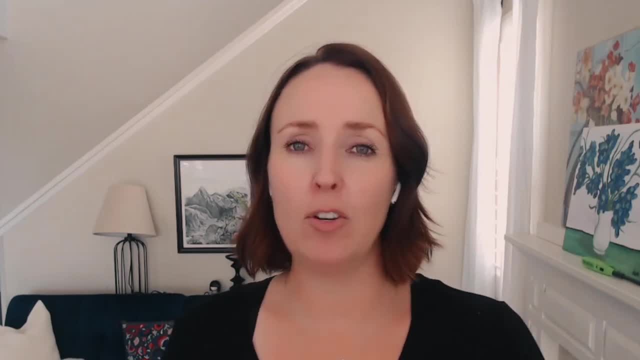 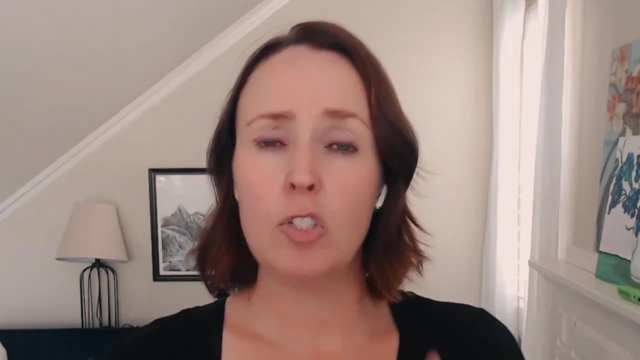 But I don't like crowds. I hate crowds actually- And so I usually avoid the tours and things that are big masses of people And I usually go towards more private tours and things of that nature. So just know, if you're going on a cruise, you don't have to do the ship's shore excursions. 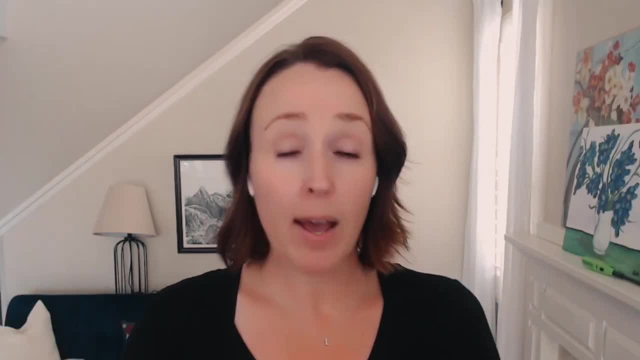 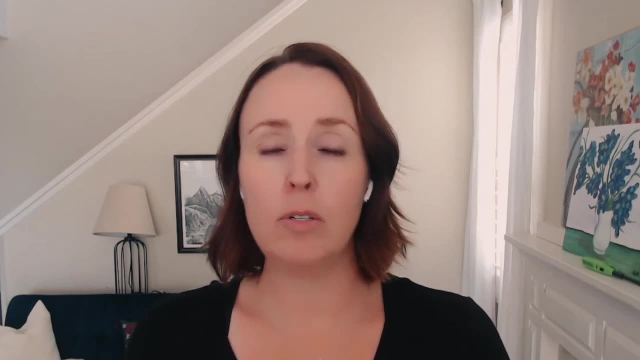 You can choose to do your own as well. Now, there's a few caveats to that that you need to know. A: you need to make sure your timing is right. You need to make sure whatever you decide to do, it doesn't leave before the ship actually arrives. And secondly, you want to make sure you're going to be back in plenty of time before the ship leaves, Because ships do not wait for guests. They do not wait, They will leave. So you want to make sure you're back in plenty of time. Also, you want to make sure that that particular port allows you. 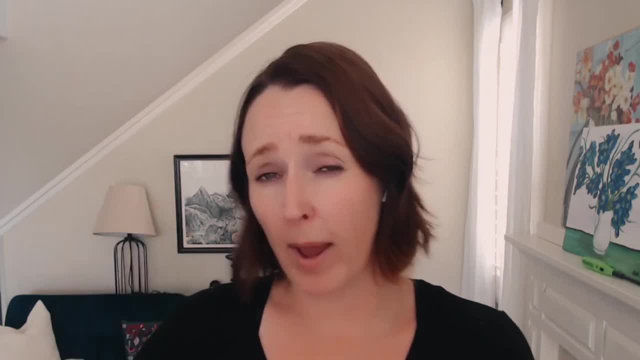 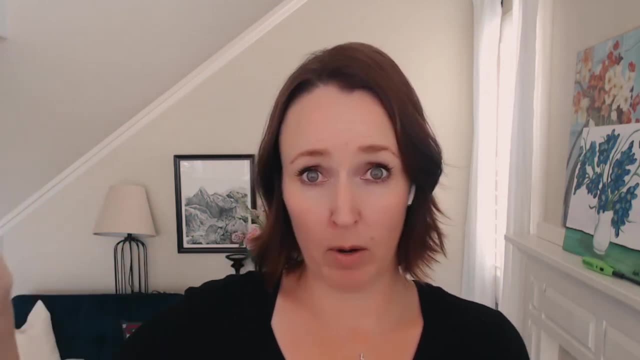 to have private things to do and doesn't require you to do a shore excursion. When I was in the Caribbean, there were some islands that you could only get off the ship if you were doing one of the excursions. So you need to check that as well, And the way you check those things is just check. 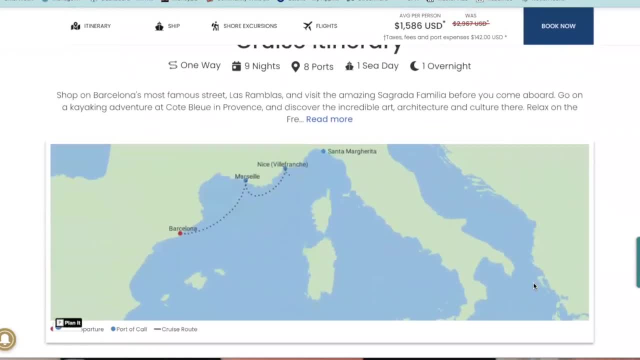 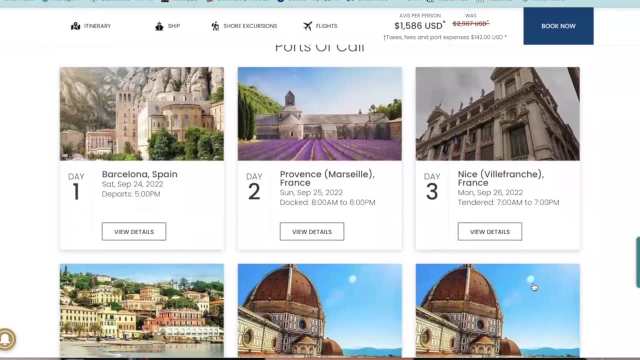 on your cruise line's itinerary. They should, for each port, tell you exactly what the arrival and departure times are, But also if there's any stipulations with regards to are private tours allowed or if you have to go on a shore excursion, or what the situation would be. 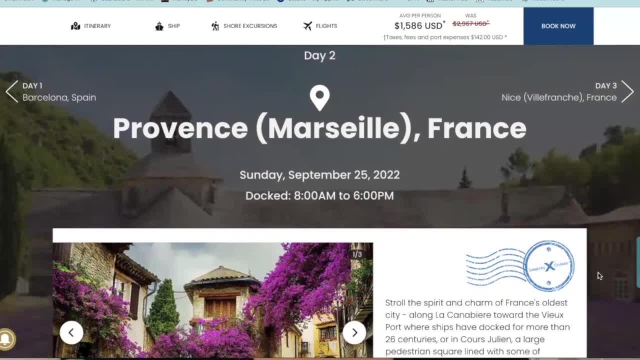 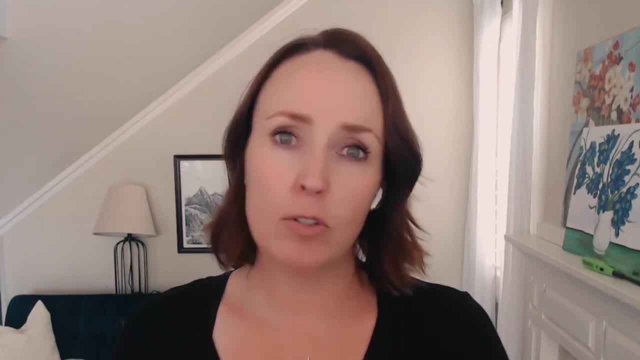 So make sure you keep those things in mind. And if you want to do something outside of the shore excursion by the ship, there are tons of places you can go to look for those things. You can either do it yourself, rent a car, do something. 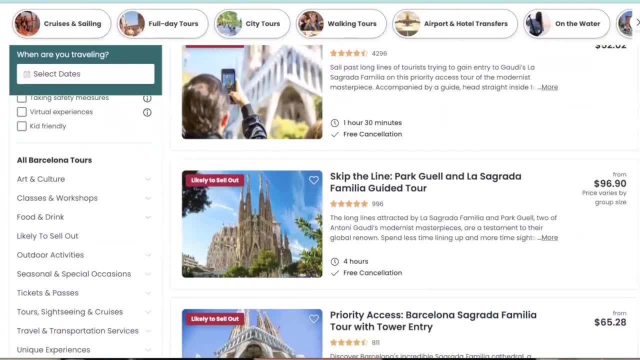 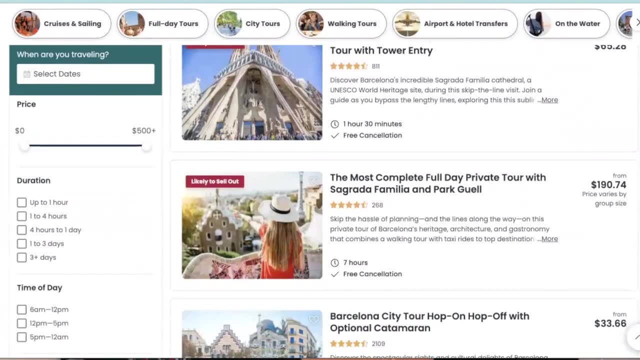 you can book something like through Viator, which has tons of tours and activities available and reviews. You can pick and choose what looks good to you. They also have a lot of private tours and things you can do, So just know you're not stuck with just the excursion though the 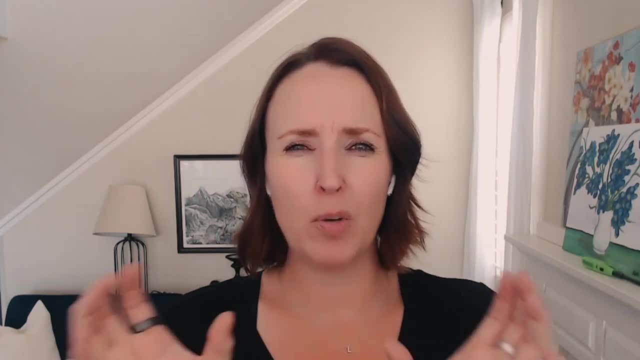 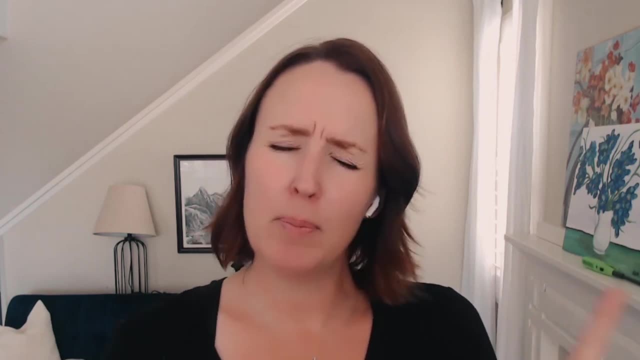 excursion is definitely a possibility for you. So it just depends on what you want to experience and how secure you want it to be and how willing you are to maybe play around a little bit. Just make sure you get back to the ship in time. They will leave, I promise. 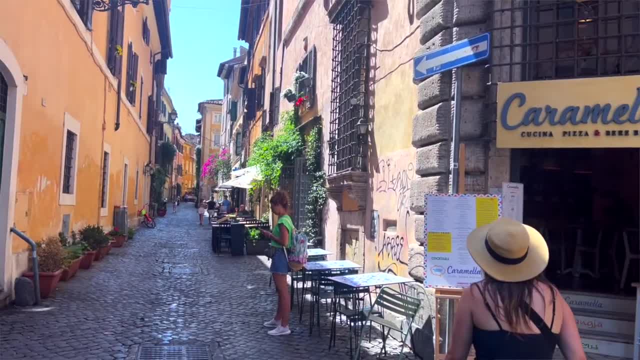 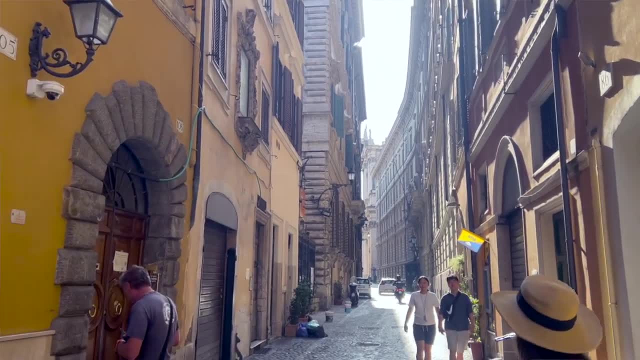 You, they will leave All right. the other thing about the Mediterranean in general, about Europe in general, is the conditions of what you can do. So if you have mobility issues at all, you might want to do a little bit more research into the possibilities in the places you're going. 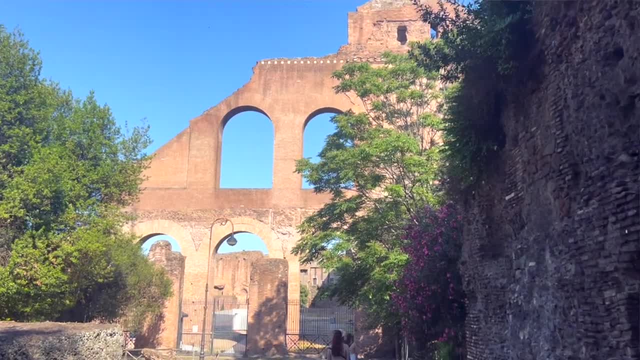 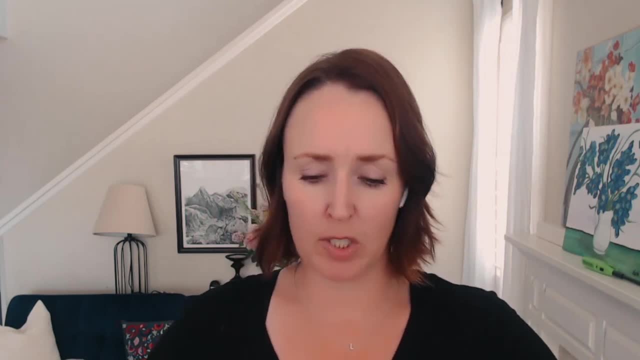 everywhere We went in our Mediterranean cruise. Most of the places were big touristy places, but it was cobblestones everywhere, everywhere, if not more. When we were in Rome, it wasn't just cobblestones. There was an area over by the coast. so it wasn't just cobblestones, There was an area. 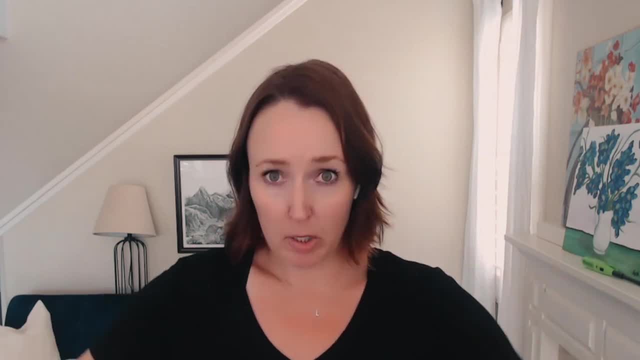 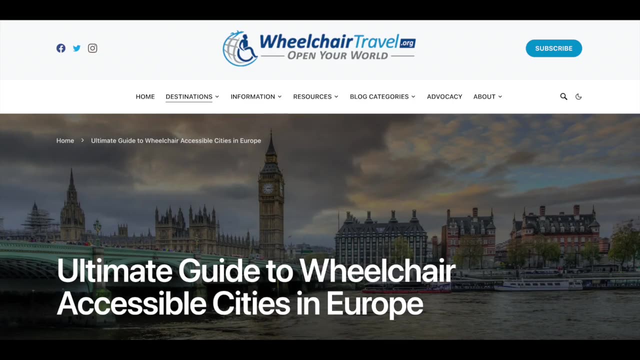 over by the Coliseum, which was actually big boulders, and so it was a little bit harder to you really needed to pay attention where you were stepping over there. so if you have mobility issues, know that going to Europe and make plans around that. now, for instance, we were in Portofino, which 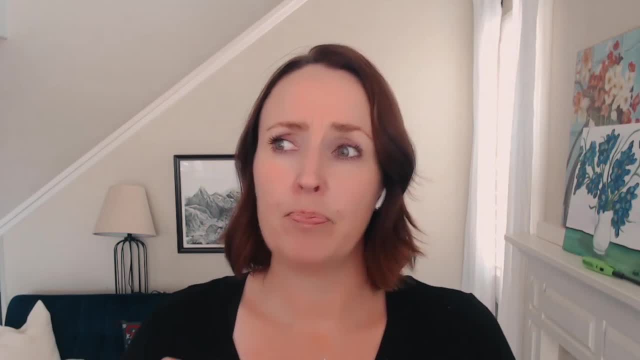 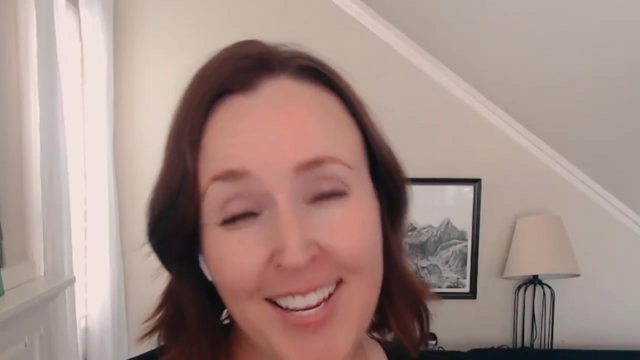 did have cobblestones and I did see people pushing wheelchairs, so it is possible. but just know that going in and know that might be an issue, but also know that, for if you don't have mobility issues for footwear, maybe don't wear heels when you're exploring cobblestones. you know what I mean. so 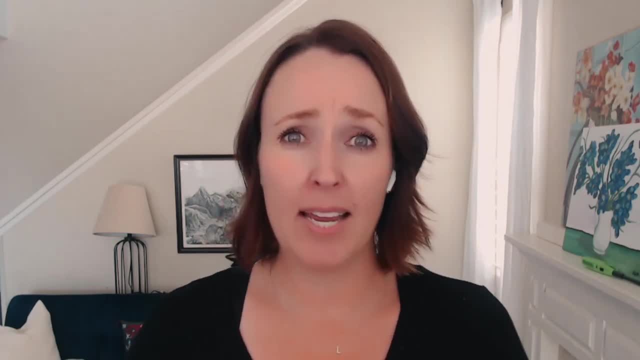 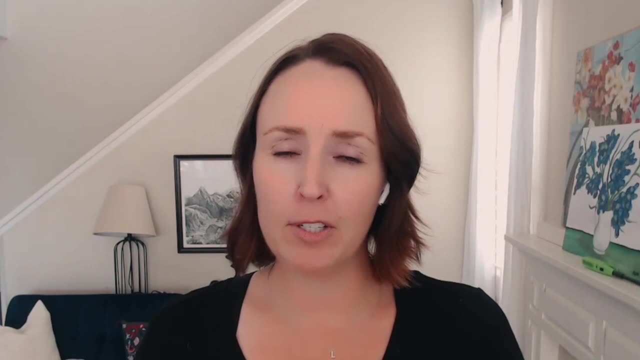 just kind of know those things ahead of time. if you're going in the summer it is hot and humid, and did I say hot because it is really freaking hot. so just know that to plan your day, maybe get off of the ship a little earlier in the day, when it's not quite as hot, or wait and go if you are. 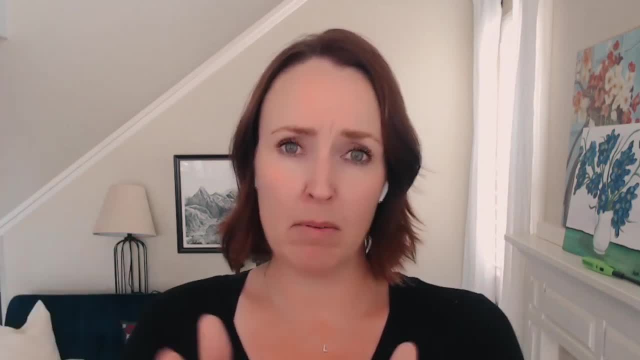 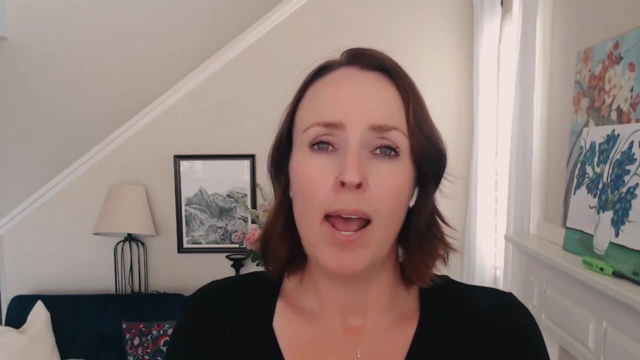 lucky enough that they're going to be staying into the evening, go back in the evening, maybe miss during the main heat of the day, which also happens to be the busiest time of day, when most people are also on shore, and just plan around that. no, it's hot. no, the roads aren't the. 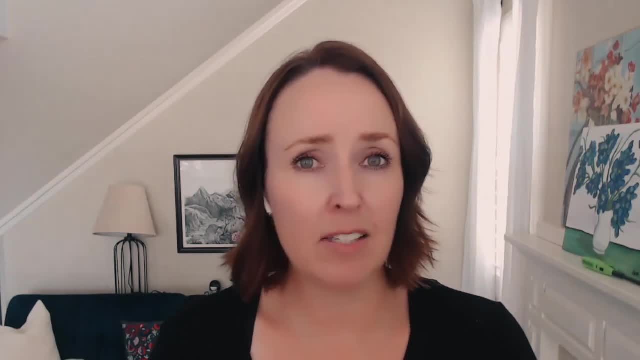 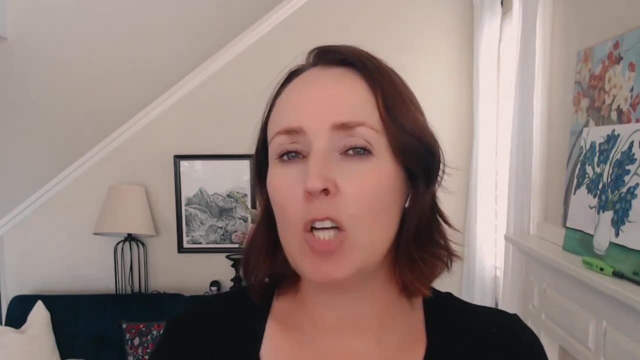 greatest for mobility there's. I didn't see elevators and things of that nature, so just plan around that, know that's going to be something and and know what to expect and have a plan for getting around it. okay, next is talking about language. now, if you're going to all of those, 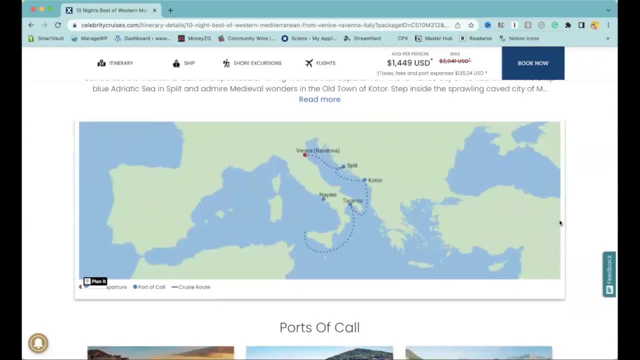 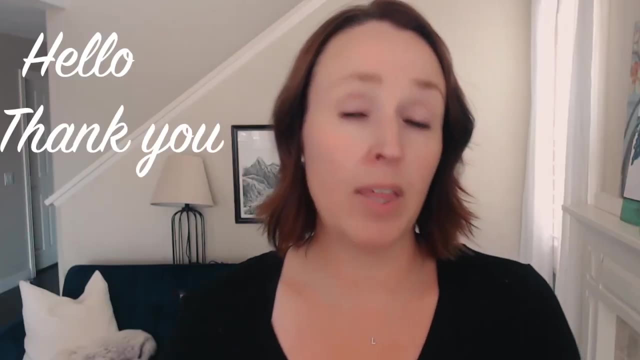 main stops on a Mediterranean cruise, chances are most of the places, at least right there at port, are going to speak English, so you really aren't going to need much in the way of language, although I still highly recommend. if you learn some basics in each of the countries, you're going to things like hello, thank you, excuse me, and even do you. 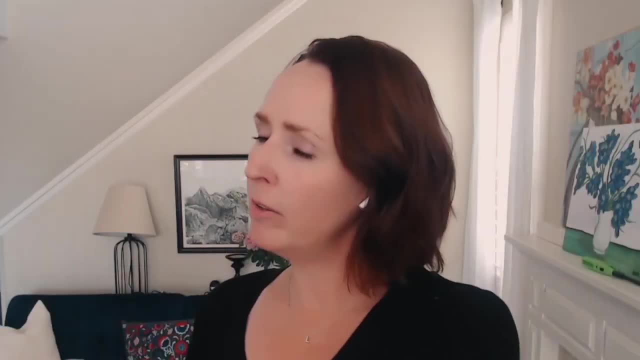 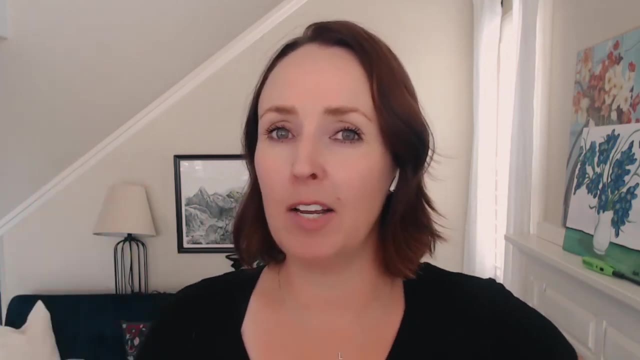 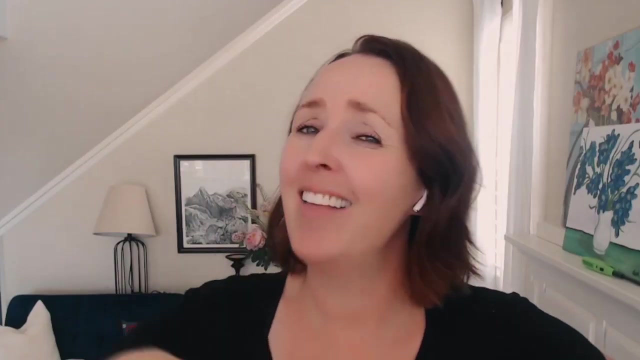 speak English, because that could come in very helpful in all the places I went to I. I was prepared to speak the language and I had planned to speak the language, but when they saw me they immediately knew I was English or English speaking, go figure. and so they immediately launched into English and I didn't even have a job. 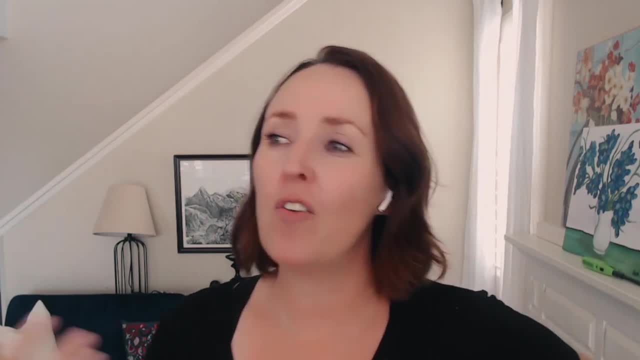 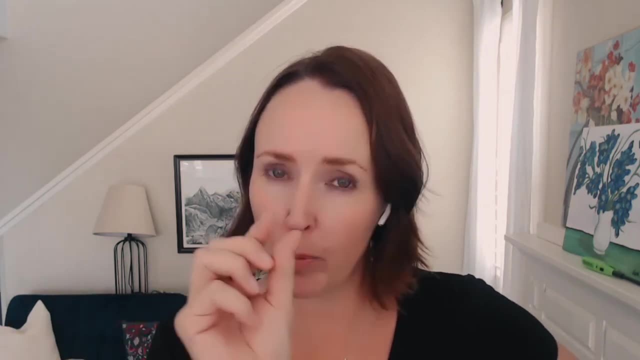 and I had no chance to try to use any of the language that I learned, so that is something that might happen. however, I did have to go to the pharmacy a few times and they didn't speak English, so the little bit that I did learn came in a little bit handy, but I was able to point in. 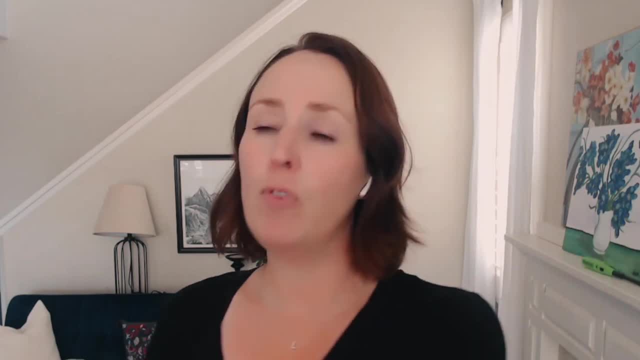 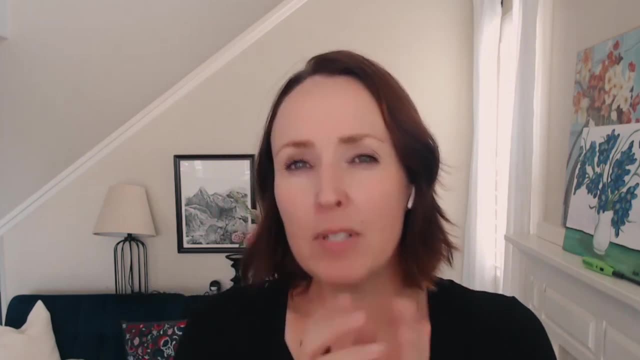 mind and we were able to figure out what it needed to do. so if you are going on a Mediterranean cruise to several countries, I wouldn't worry about the language too much. again, if you can learn a couple smattering of things, just to be polite, and you know, say thank you in their language. 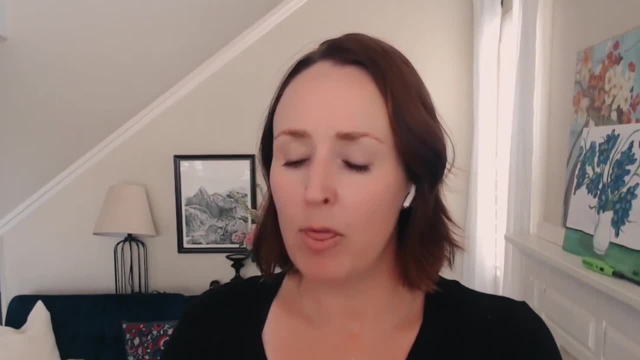 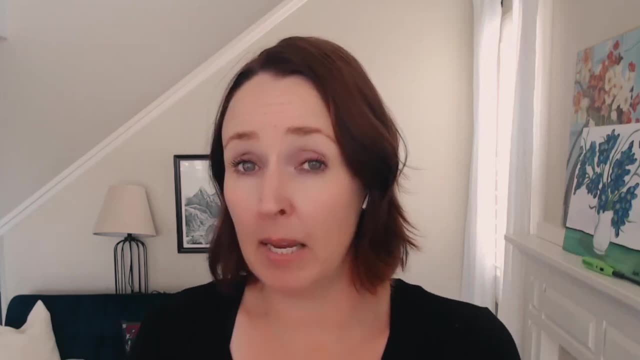 and I welcome you to it. but for the most part you don't have to worry about it. those big cities usually have a lot of English speakers, especially at the restaurants and the shops where they're expecting tourists to be. if you go outside of those big tourist areas- the ports, where the ships 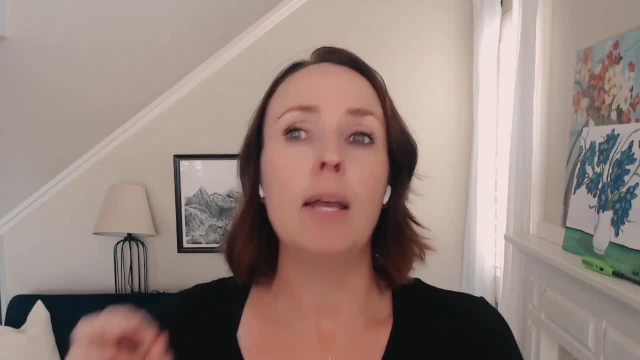 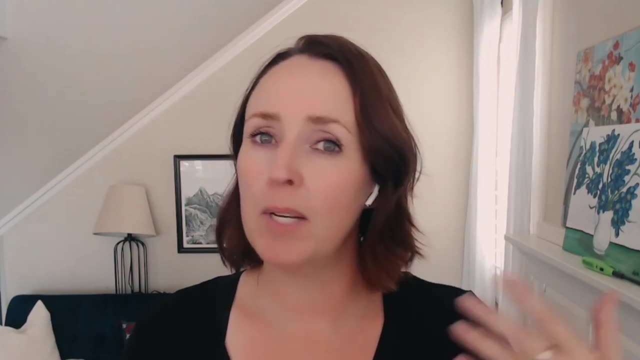 drop off at you might find a little less English. so if you know part of you, what you're going to do is to explore a tiny town, say in France. then maybe learn a little bit of French, because you don't know if they're going to be able to speak English and you'll want to be able to do at least. 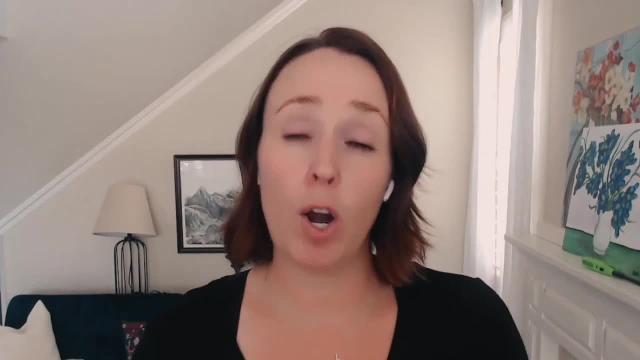 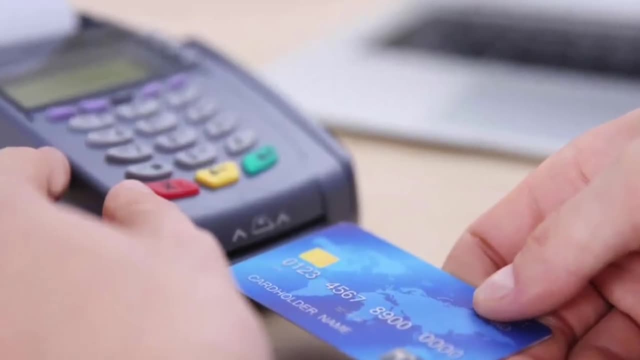 minimum of communication when you're there, all right. my next tip is regarding money. now again, most of those main tourist areas are going to take credit card. they're going to expect tourists to use a lot of credit card, and so I highly recommend having a good card that does. 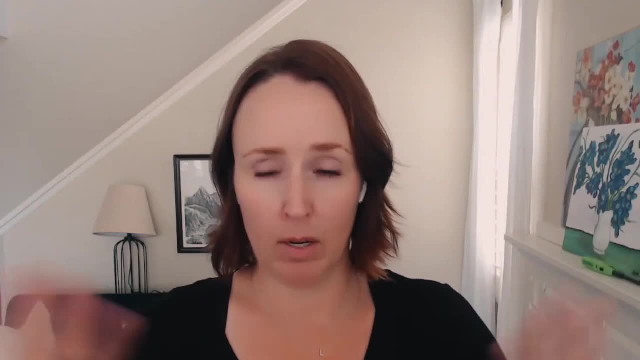 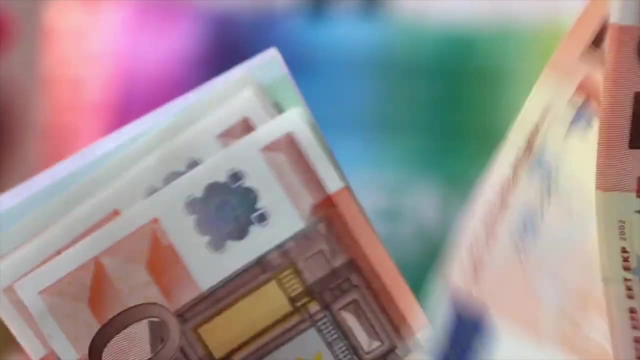 not charge foreign transaction fees. you know that you feel safe using in a foreign country cash. though, although you don't ness like you could get by without cash- you don't necessarily need it- I still highly recommend you have some euros, because there are going to be times when it was. 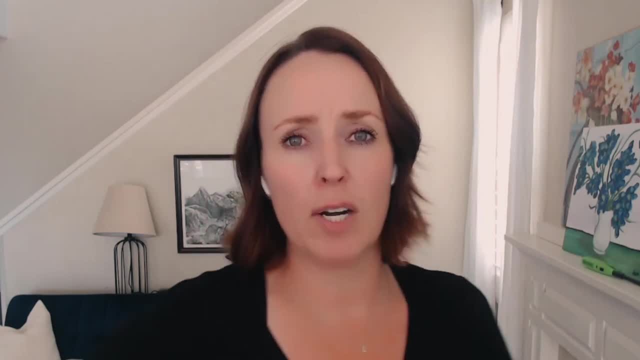 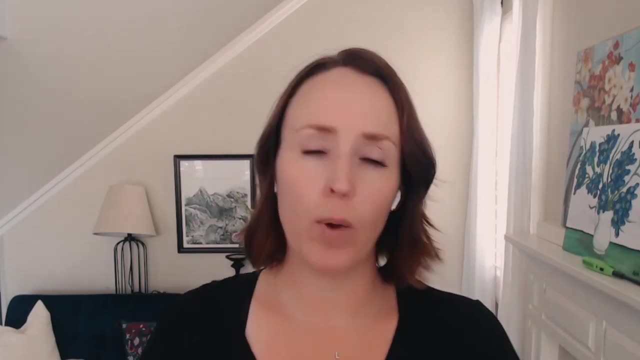 far easier to give a euro than it was to try to dig out the card and ask if they took credit card so you know if you're buying a bottle of water or buying a gelato. it was just way easier to have cash to pay for that than trying to worry about credit card. so I would highly recommend having 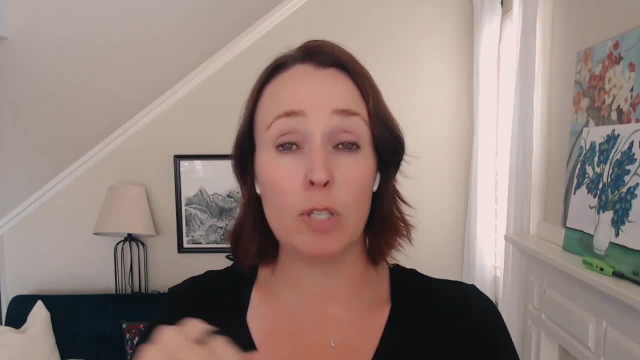 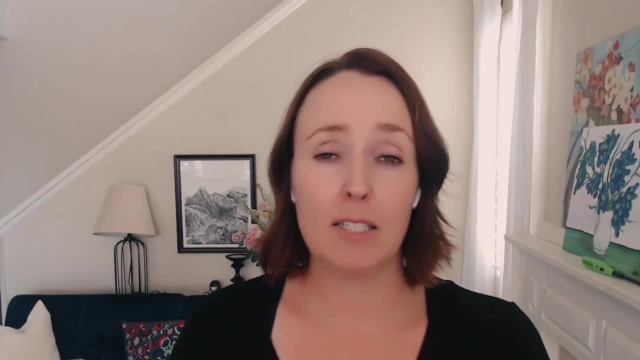 a little bit of cash with you. also a lot of places if you need to use a public restroom. they're not just available for for everybody, so you might want to have a few euros in case it's a paid toilet. you might need to be able to pay in Italy. 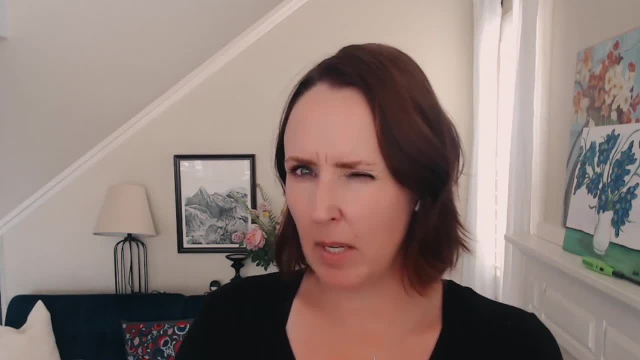 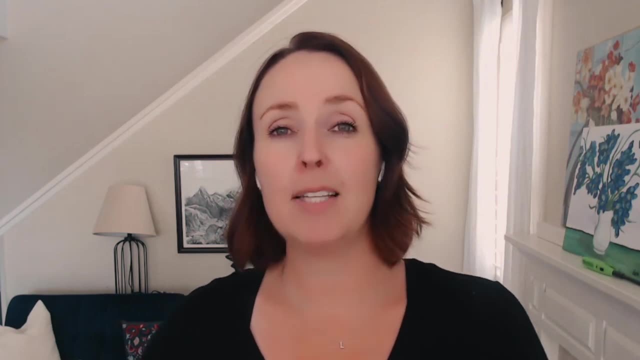 That is definitely a thing where you would need to pay to use public toilet. And then, speaking of toilets, you also want to know that they're a little different than what you have at home. When we were in Rome, some of the toilets that we went to- public toilets that we went to, for instance- don't have toilet seats. 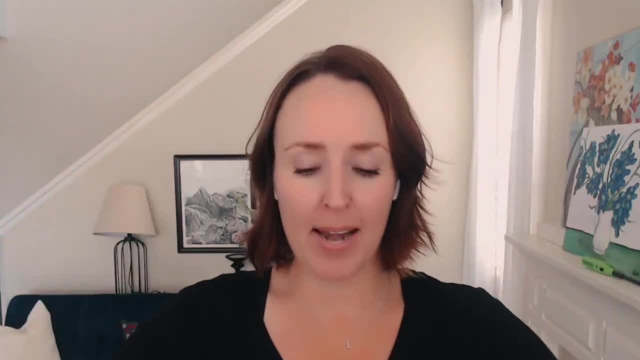 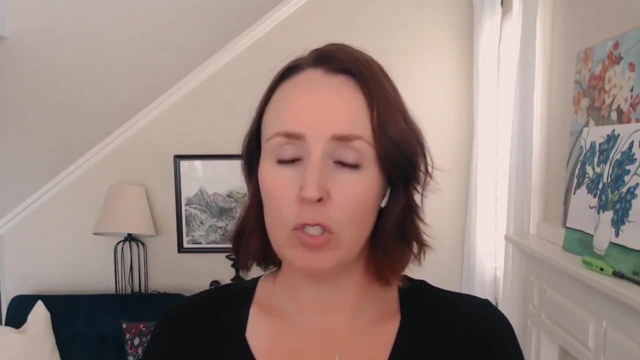 Just know that's a thing. Also, the way they set it up it might have a gender-neutral washing area and then separate toilet areas for men and women. But just know so you don't freak out if you walk in and see the opposite sex standing there. 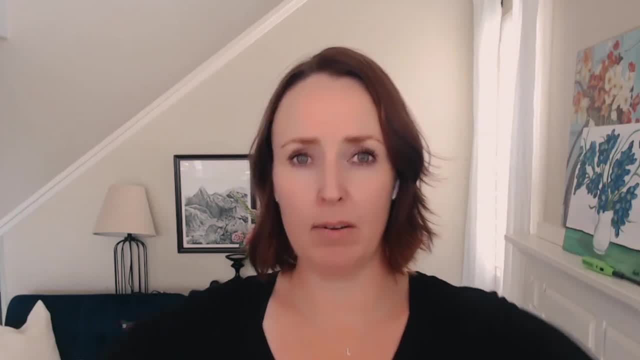 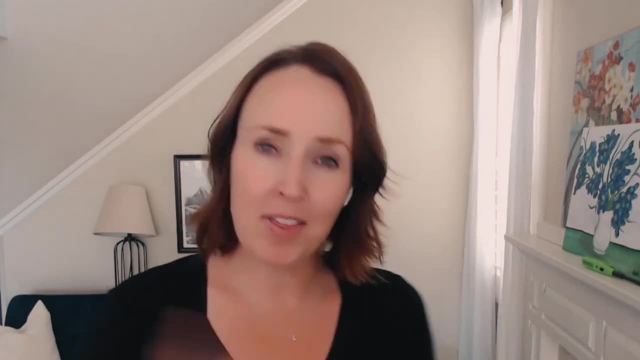 It's sometimes a gender-neutral area and then toilets are separating. after that, All right, and then my next tip has to do with food. So one of the things I always dreamed about going to Europe in general was I wanted to explore the food. 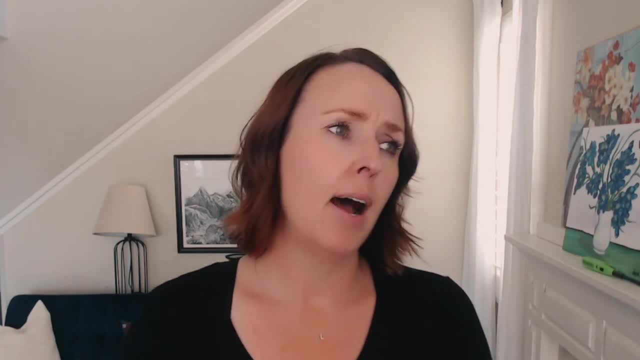 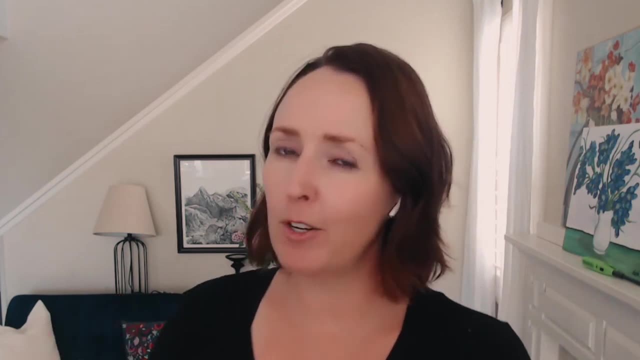 And I thought the food would be so much more amazing than what we get in America. I don't know why. I just assumed that everything is fresher and doesn't have all the preservatives that we have, And so I was really looking forward to the food. 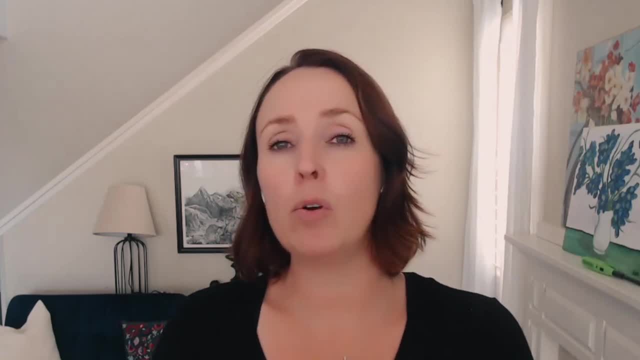 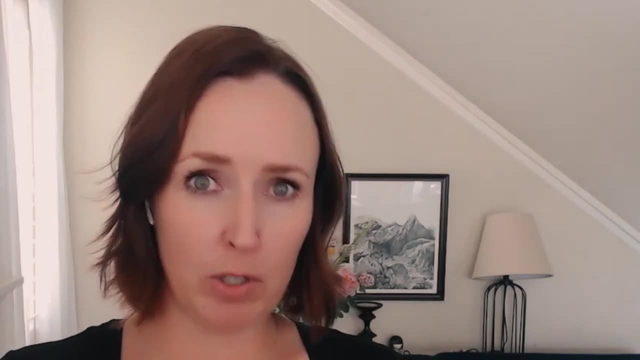 And I think that's true in general. But when you're in the main touristy areas and you're going to the main touristy restaurants, that's not always the case. I'm sure the food is way fresher than what we have here and chemicals and things like that. 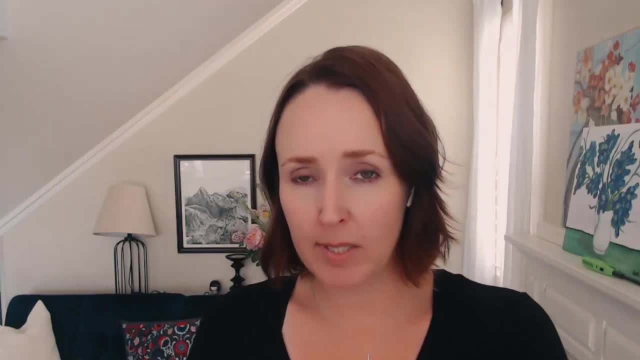 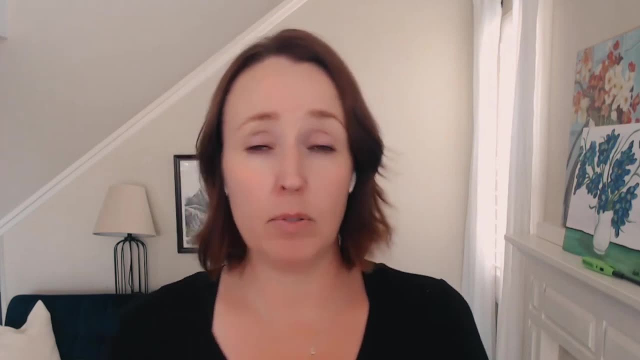 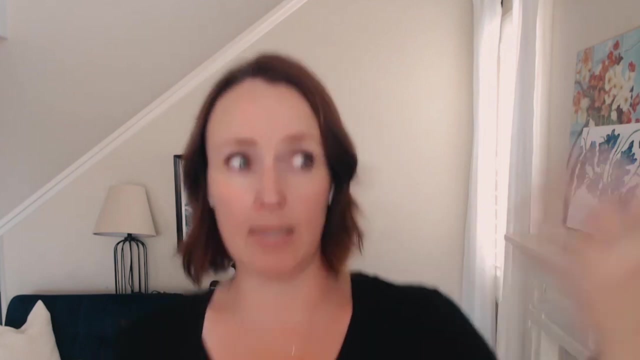 But the actual food quality when I was in a touristy restaurant honestly wasn't much better than anything that I can get in America. It was pretty, it was good, It was fine, It was good, But it was kind of standard for what I would get in America if I went to, say, an Italian restaurant. 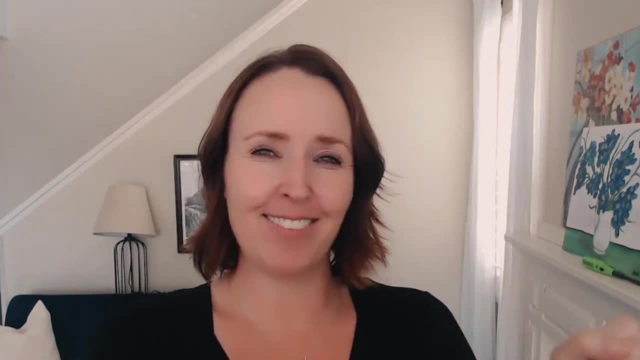 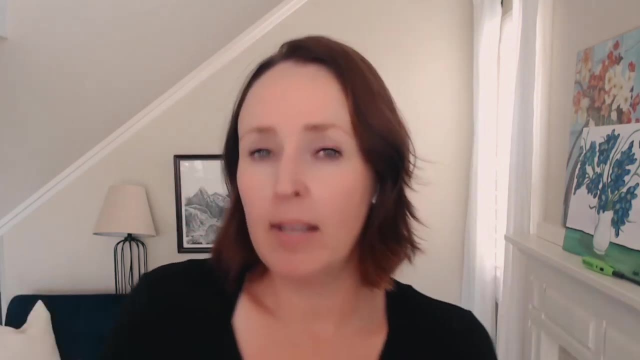 Like a good- I'm not talking Olive Garden, I'm talking a good Italian restaurant in America. It was about what I got in Italy, Same thing with France and with Spain. It was like it was okay, But I was primarily in those touristy areas. 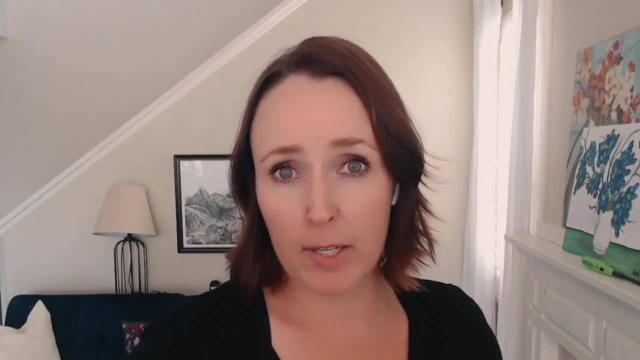 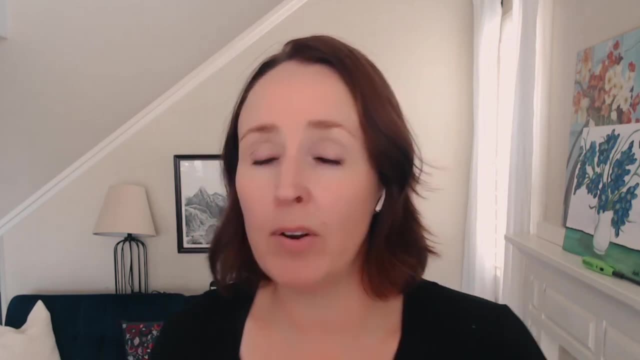 I think if food is something you really want to explore on your Mediterranean trip, if you just go to those touristy areas, I think you're going to get disappointed, Unless you happen to live in a really small town that has terrible Italian food or French food. Then you might be happy. But if you live in A town that has decent restaurants of those type of cuisines, then you might be disappointed only going to the touristy areas. So if you're a foodie, I highly recommend you do some research ahead of time. 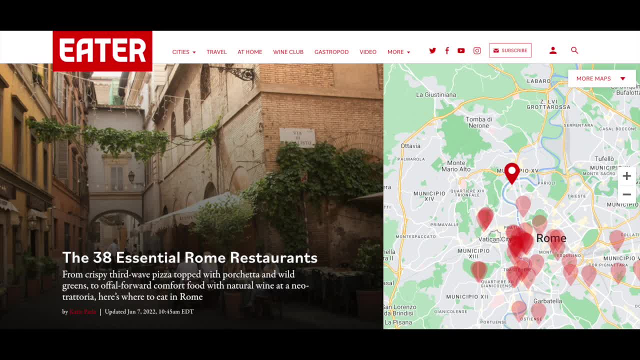 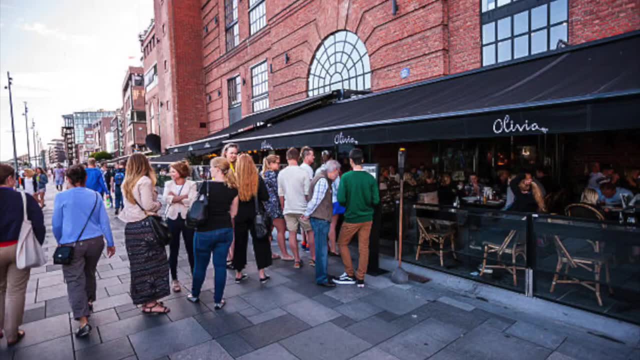 And either A- look up the restaurants and know where you want to go and just go there. Don't show up and expect you're going to just find one. So research ahead of time. Or B- look for lines. If there's lines, chances are it's good food and it's worth the wait. 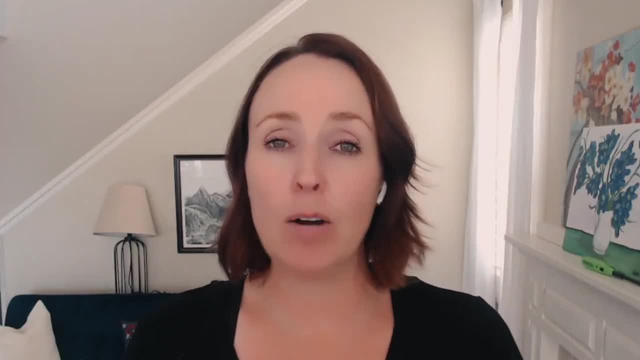 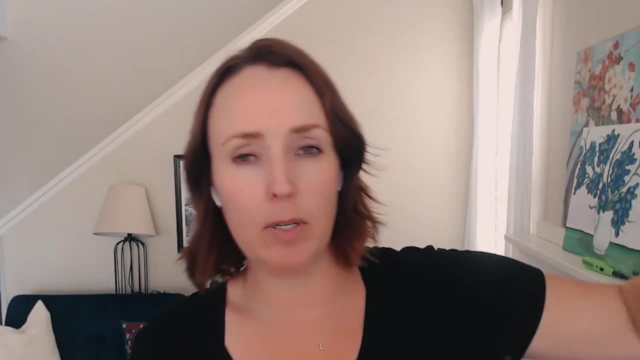 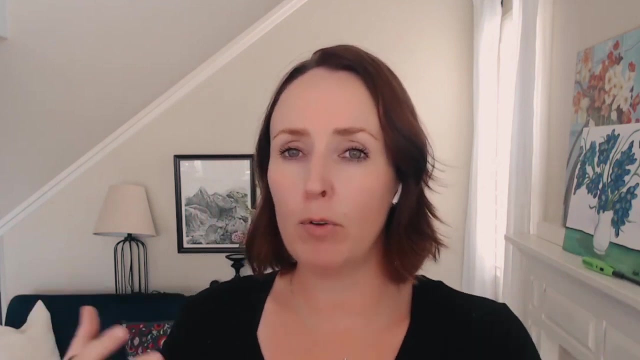 Or my last tip for that is to get outside of the touristy areas. Go to a little small town away from that main area. Go outside of the main neighborhood, maybe travel a little bit away. Chances are, if you get away from the touristy areas you're going to find far better food quality and more home cooking, things of that nature. 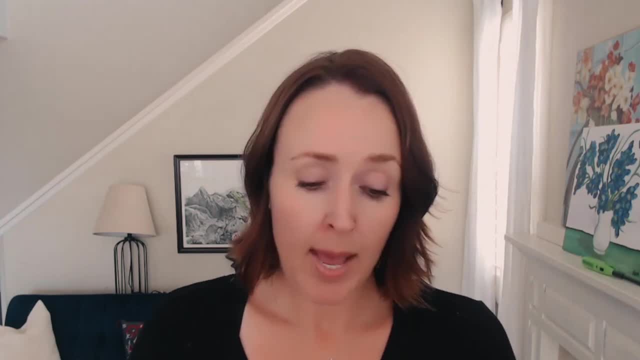 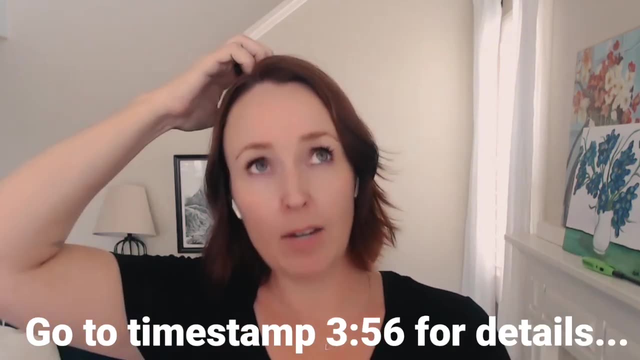 But remember, know a little bit more of the language if you're going a little farther away and they may or may not take credit cards, So make sure you have cash, All right. My next tip has to do with flights. Now I already talked about checking with your cruise lines flight department. 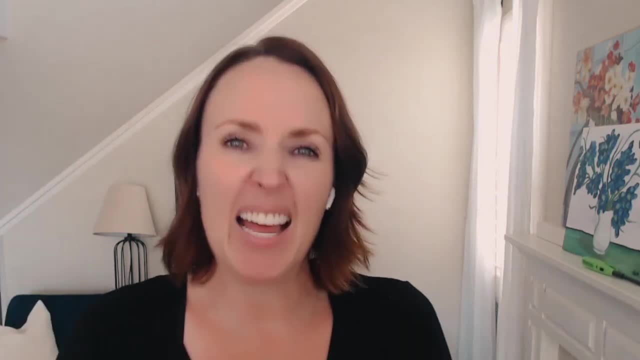 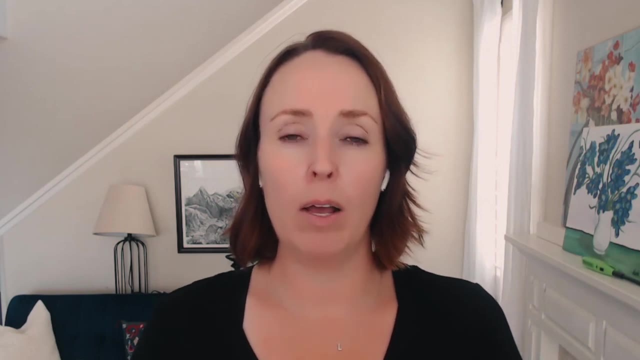 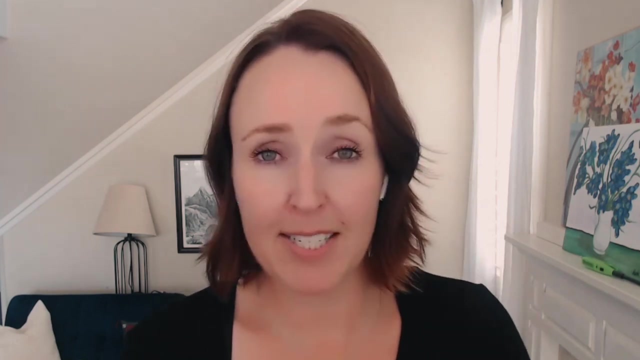 But with regard to To the flight that you actually booked, I highly recommend, if possible, pick a direct flight, just because, again, if you're coming from far away, that is a very long trip and it would be nicer not to have a large six hour layover, for instance in the middle of it, and just get there quicker. 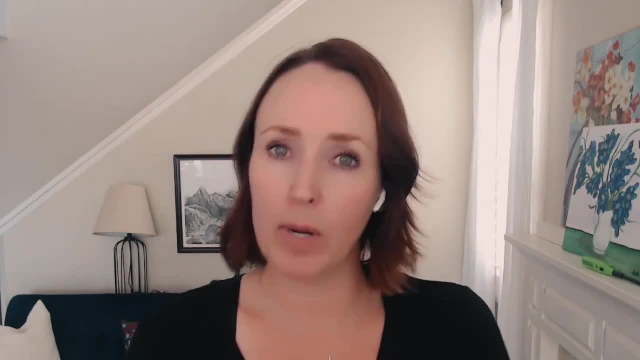 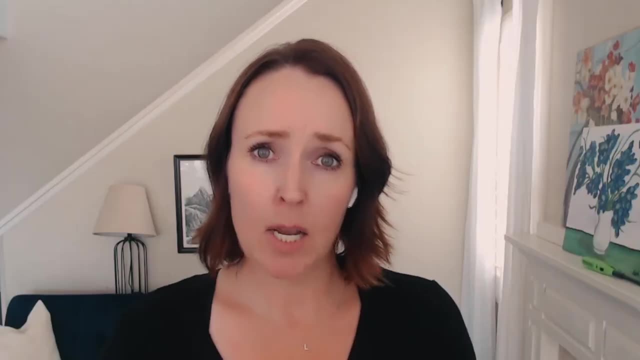 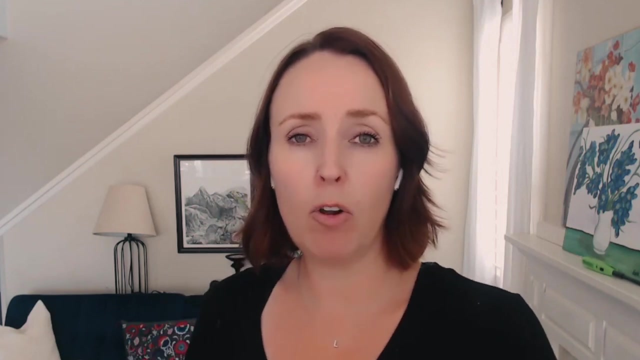 Secondly, if you can afford to do so, I highly recommend upgrading your seat, whether it is to the premium or to business or first class, if you're fortunate enough to be able to upgrade to that, Or use your credit card points to upgrade, or if you have upgrades through, say, if you belong to the airlines membership program, if you can get upgrades that way. 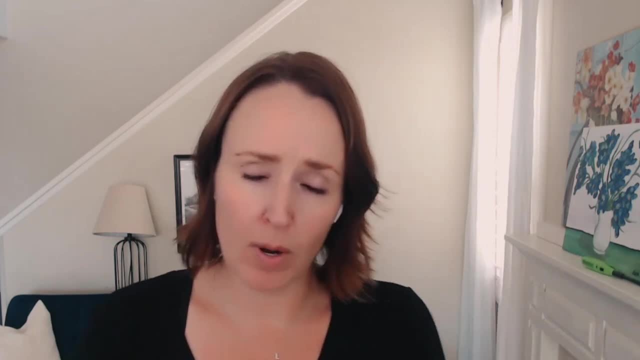 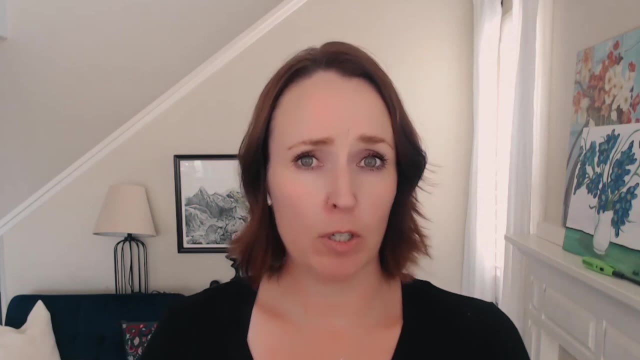 I highly recommend, if you're going that far, do everything you can to upgrade your seat, because you will be far more comfortable than sitting in the coach seats, which can be torture after a 10,, 12,, 20 hour flight. So definitely do those things. Also, if you do happen to have connections, make sure you're building In plenty of time. I don't mean one or two hours, I mean a lot, especially if your first stop is in a foreign country. So, for instance, we left from Los Angeles. Our first stop was London, So in London we had to go through another TSA line with their version of TSA, which I don't understand why we had to do that, since we already did TSA when we got on the plane, But we had to go through a TSA line. 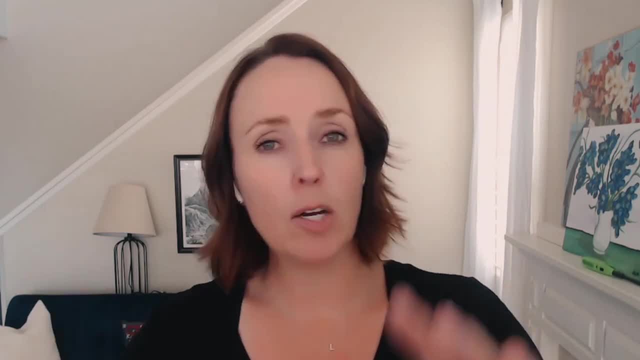 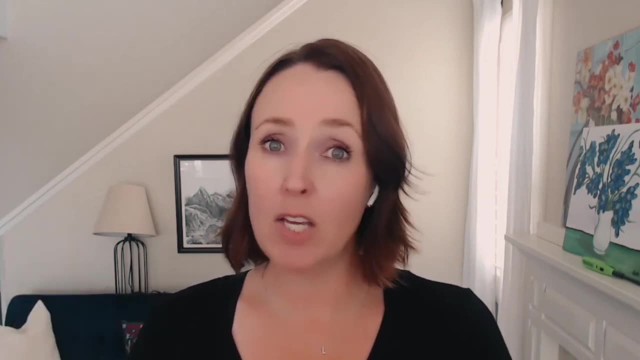 We had to show our passport. We had to go through an entire rigmarole To be able to get through. Plus, Heathrow in London is ginormous, And so it might take you 20 minutes to get to your next gate or terminal, things of that nature. 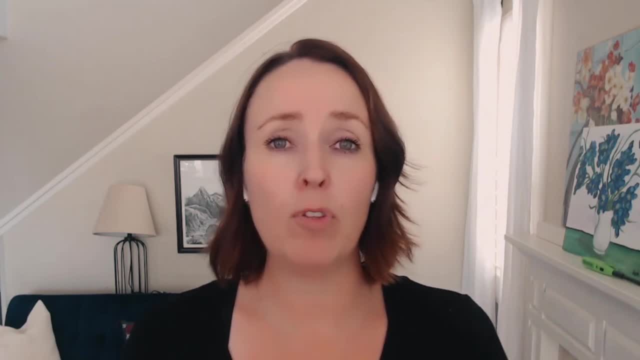 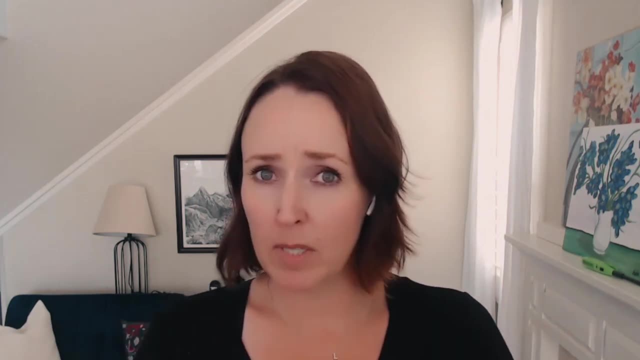 And it's not just at Heathrow. There are other countries too, even if they're a smaller airport. Usually, if your first stop is a foreign country, there's going to be some sort of passport control customs type of a situation that you're going to have to go through. 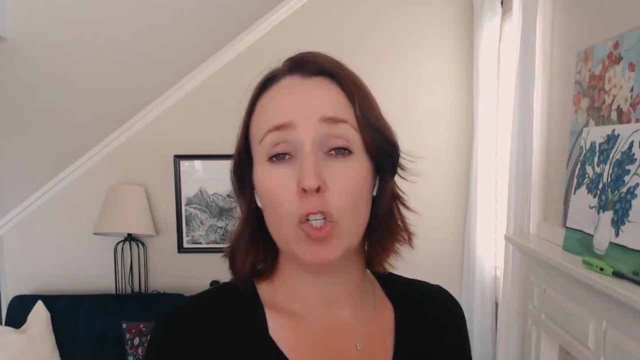 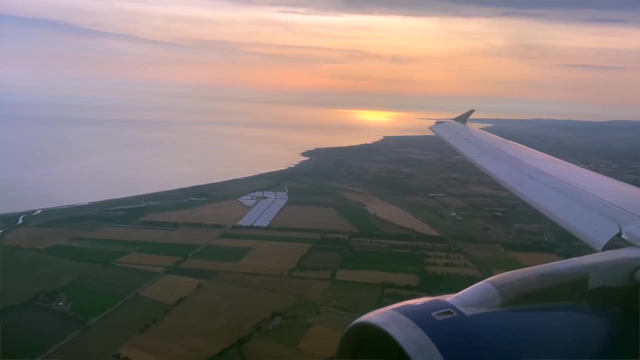 So make sure you're building in that time. This also protects you in case your flight is delayed for some reason Or canceled or something happens- to protect so that you can catch your next flight. So make sure you build in plenty of time in those. 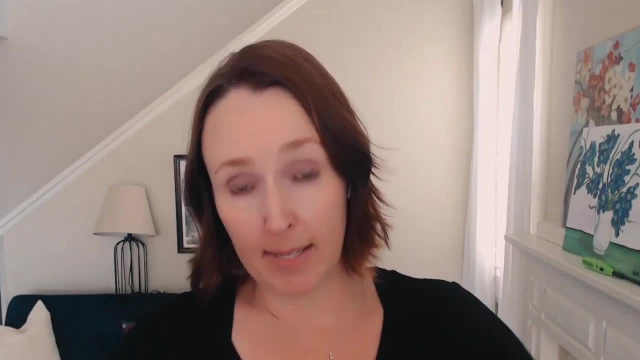 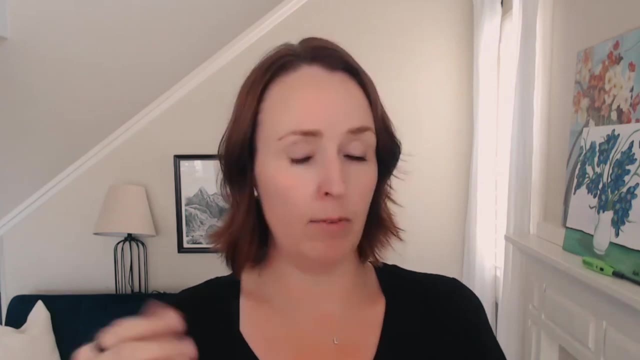 If you find yourself with six hours of time, like we did in London, then consider using some of the first class lounges. Now, you can either do that because you happen to be flying- obviously business or first class- but you can also get it through your credit card. 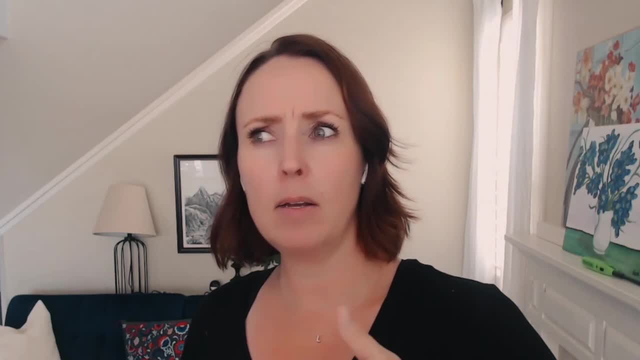 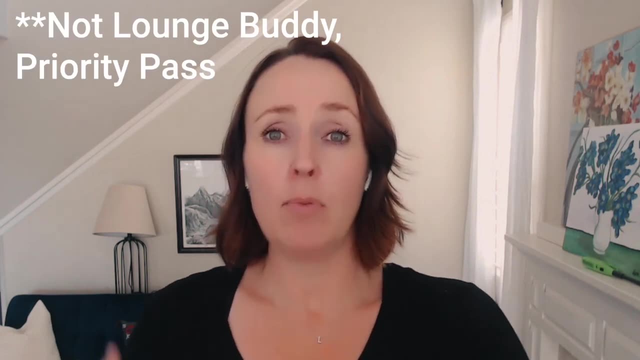 A lot of credit cards is like if you have Amex, they're platinum or they're higher level credit cards and some of the others. We'll offer lounge access or lounge buddy access that you can get through that or again through your membership of your airline. 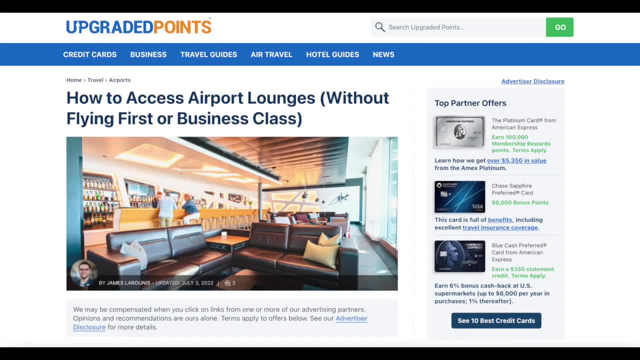 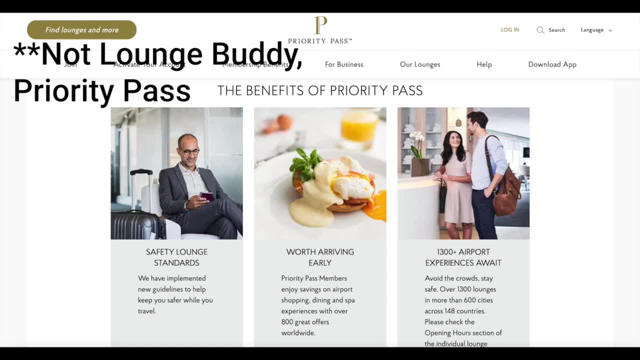 The other thing you can do is consider buying a day pass which you just gives you, like for $30,, say you have access for the whole day. And then also there's a third party lounge systems like lounge buddy, which gives you access to over 1600 different lounges worldwide. 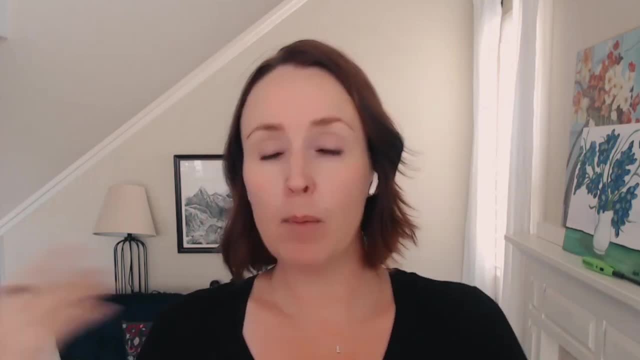 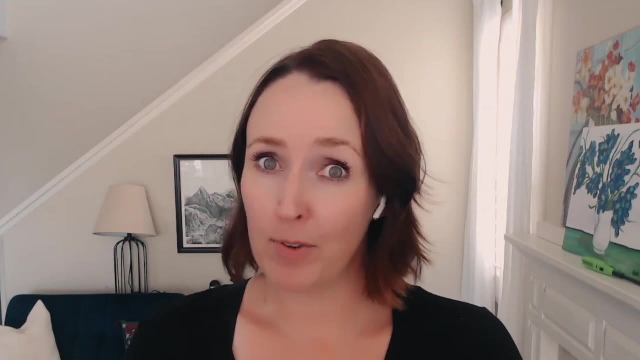 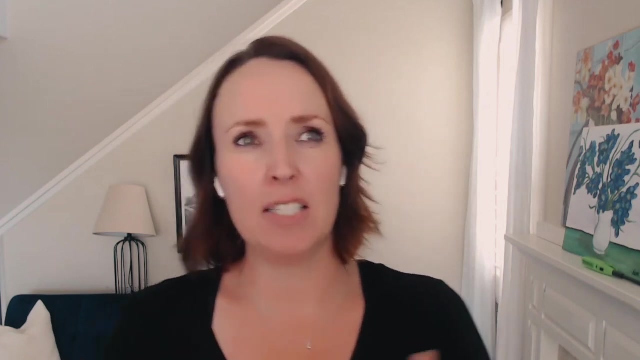 You just want to make sure there's one of their lounges where you're going before you buy their membership program, But that's also an option as well, just to make that stay or that wait a little more comfortable. And then my final thoughts on the flights is make sure you don't, and actually isn't so much the flights.